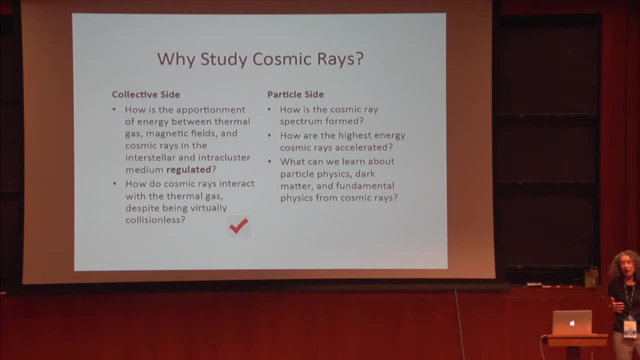 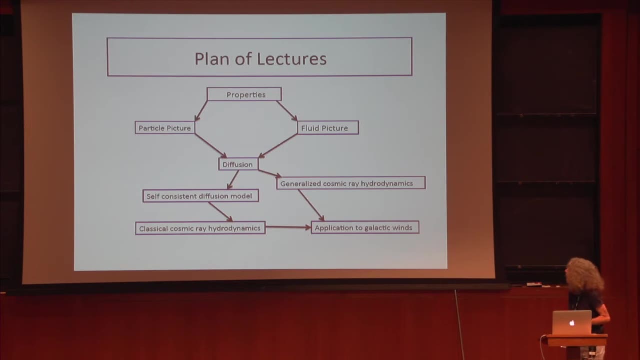 fundamental physics from cosmic rays, because they do represent the highest energy form of matter that we know and can work with. So here's sort of a flow chart- since this is computational plasma astrophysics- for how I'd like these lectures to go. So we're going to start with some slides, where I'll show. 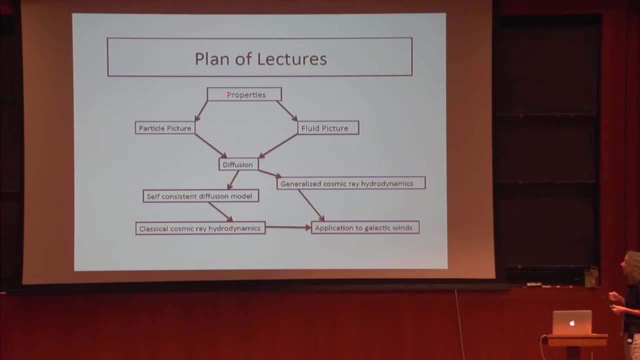 you the properties of cosmic rays, and then that will sort of bifurcate into the particle picture, which was the right-hand column of the previous slide, and the fluid picture. And I've put the particle picture here because we're going to talk about that first And 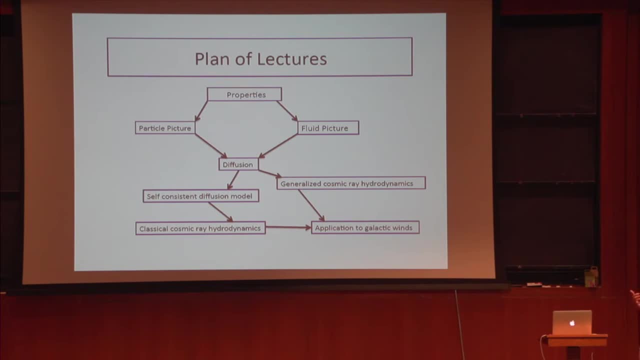 in order to understand both of these, we'll have to talk about diffusion, And then there'll be another bifurcation. So there's a self-consistent form of diffusion, which is sometimes called self-confinement, and we'll establish the groundwork for that. 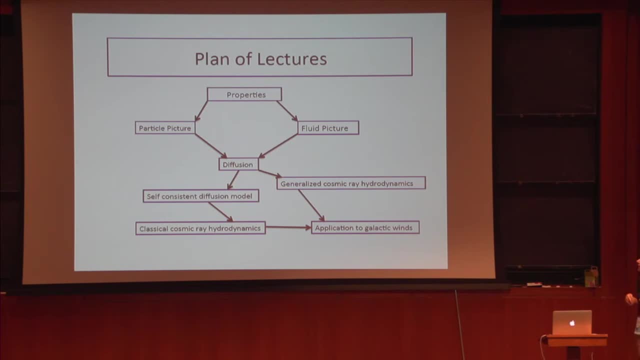 but I think not today, And that will lead to what I call classical cosmic ray hydrodynamics, which is a fluid theory for cosmic rays and how they interact with the thermal matter. But without appealing to the self-consistent model, we can just go back and look at the 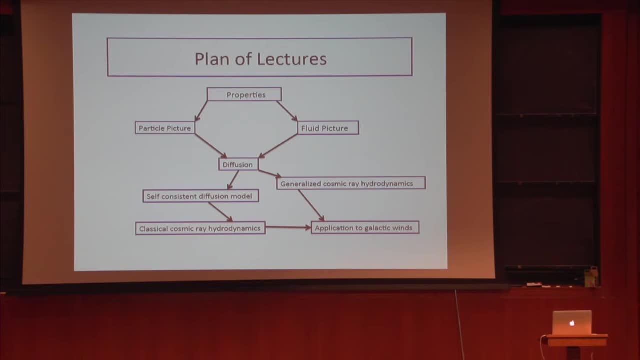 sixth principle. So what does this mean? The first principle is that the cosmic rays are the ones that are the most important particles in the cosmic environment. These are the ones that are the most important, And the second principle is that they're the most important. 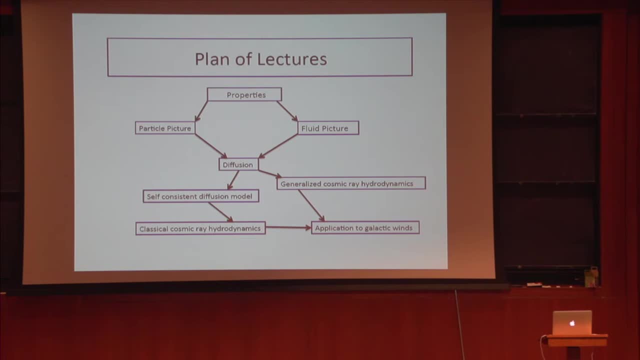 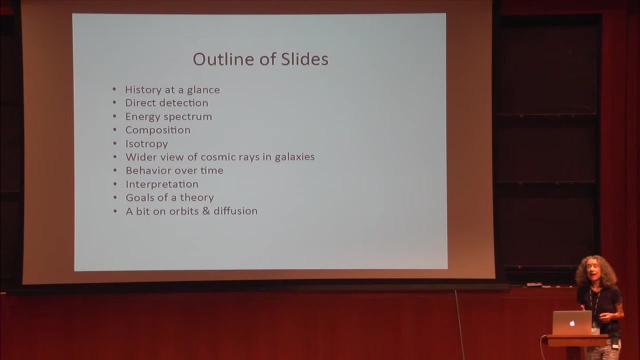 particles in the cosmic environment, And so the first principle that I'm going to talk about is the fact that the cosmic rays are the most important particles in the cosmic seen. something about galactic winds at this school will be that cosmic ray treatment matters. it matters quite a lot, and I'd also like to say that you should. 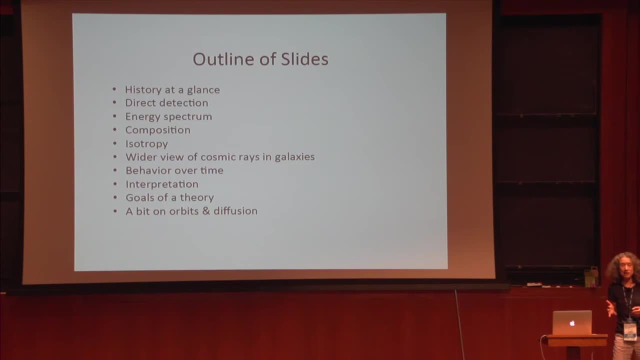 feel free to interrupt me at at any time if you have questions. I know you all have different backgrounds. I'll try to make this as jargon free as possible, but one can never succeed. so what we're going to do today is is go through some slides- things that are best shown as slides- and then the rest of it will be. 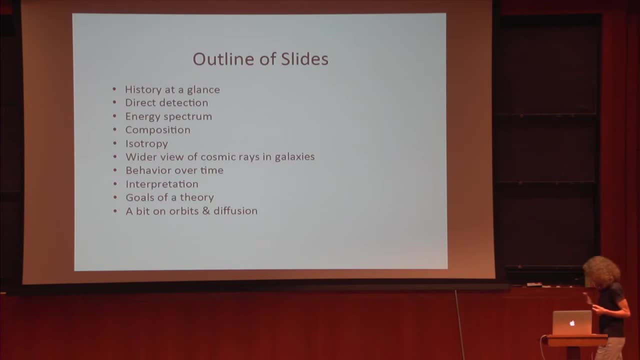 blackboard stuff and I'll show you some of cosmic rays greatest hits: how we can derive a spectrum, a little bit about Fermi acceleration, a little bit about diffusion, how we derive a Fokker-Planck equation, and then I'll apply that to the. 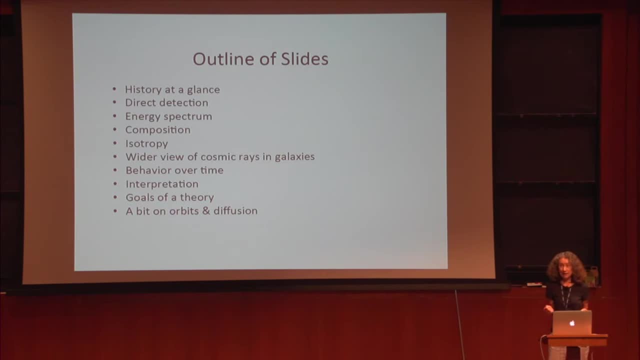 sort of first plain vanilla theory of diffusive shock acceleration, you. so that's, that's the goal for today. so this really will be a glance. the history, how we directly detect cosmic rays, then what the energy spectrum is, and the composition and the isotropy of the earth, these are all important clues that 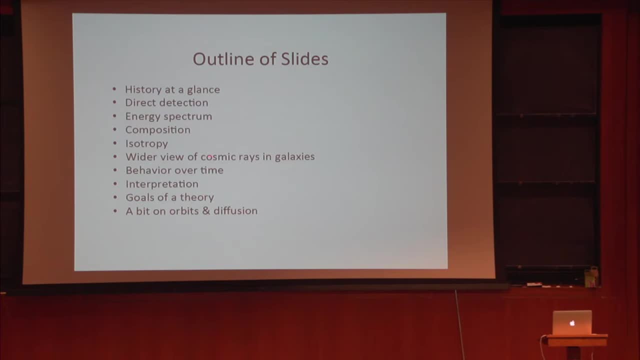 have helped us unravel what cosmic rays do in the galaxy. we can now do something more with cosmic rays in other galaxies. we can say something about cosmic ray properties over cosmic time. interpret all that so a lot of what's happening at the current point of our time as we're 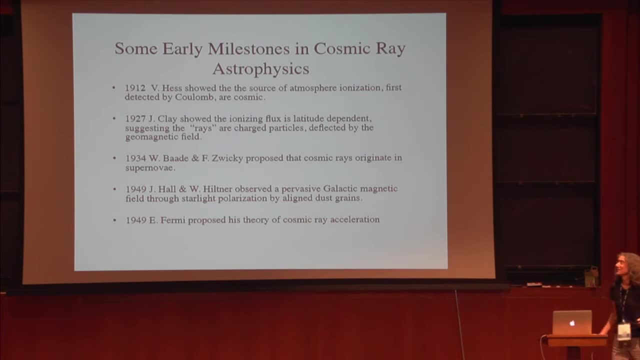 doing in the radiation review and we can start to talk about what are the most important elements we need to know about what a theory should set out to do, and then we can use what we've established so far to talk a little bit about orbits and diffusion. okay, so, um, here's the history at a glance. um, so it. was known already in the time of coulomb that there's a source of atmospheric ionization. so, at the temperatures of air there, simply aliens. but there are a few, and it was thought to be sure that the not Previously, somehora, eighteen hundred one hundred million namedсл of time, of removing meters of Lunchjust, it suffered so that caffeine belowivolierra's. 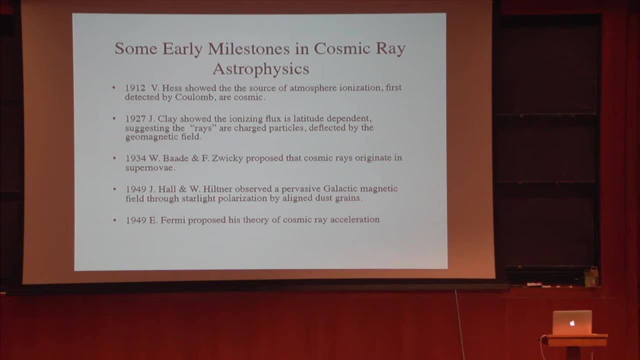 for a long time that the ionizing radiation comes from inside the earth, But in 1912 Victor Hess ascended in a balloon and showed that atmospheric ionization actually increases with height, and that was unambiguous evidence that the source of ionization is cosmic and 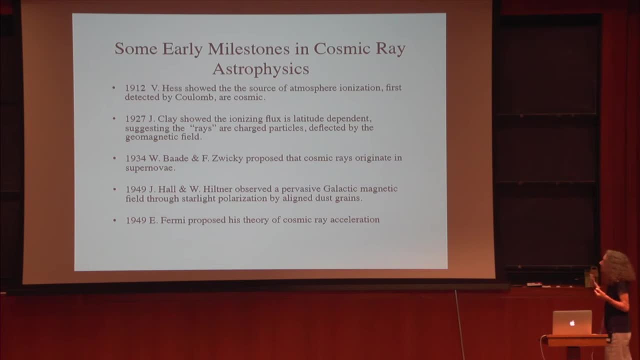 not knowing what the source actually was, people started to call it cosmic rays, And then, in 1927, it was shown that the ionizing flux actually depends on latitude, and the most straightforward explanation of that is that cosmic rays are charged particles that are bending, being bent by the earth's magnetic field, as opposed to photons, which could also 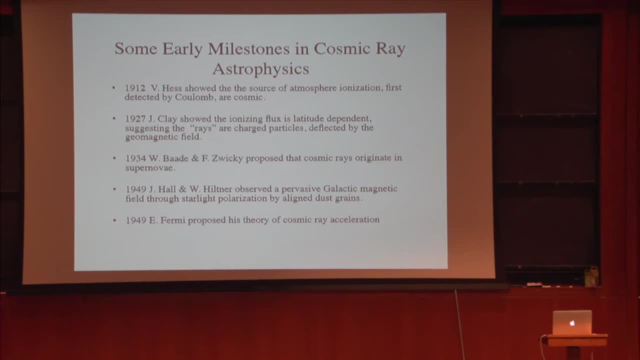 produce ionization. And then in 1934, in a crazy or brilliant leap of speculation, Bada and Zwicky proposed that cosmic rays originate in supernovae. They didn't have a detailed explanation for how, but they thought that supernovae probably were the source of cosmic. 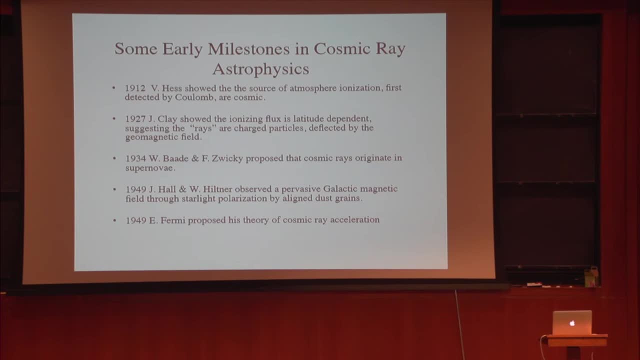 rays, And we'll see that in a way they were most likely right Then. in 1949 the galactic magnetic field was discovered through starlight polarization. That was worked by Hall and Hiltner. The dust brain alignment was predicted by Chandrasekhar, and in the same year Fermi proposed his theory of cosmic ray acceleration. 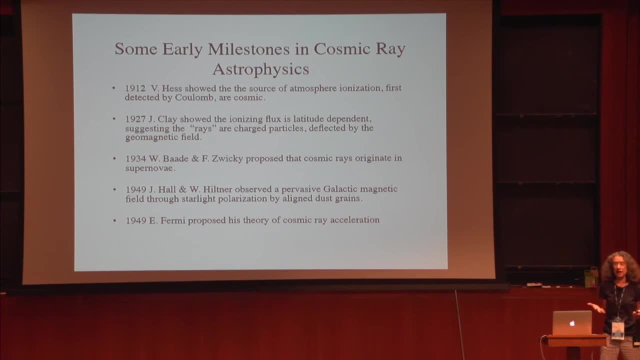 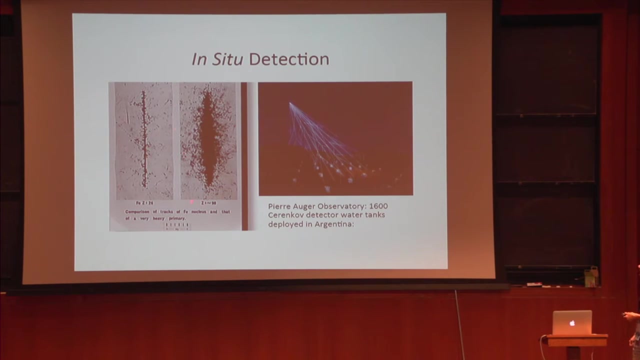 which is the sort of longest surviving theory of cosmic ray acceleration. So really by the middle of the last century the elements were in place for what became cosmic ray astrophysics, And so here's a little bit about how cosmic rays are actually detected. These are the 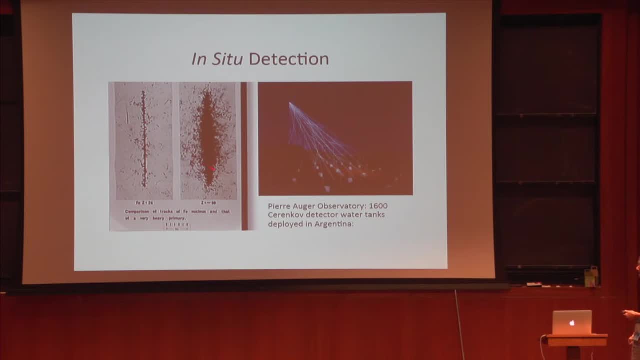 particle tracks in lexan plastic showing how you can tell something about the composition of cosmic rays: A thin track for a low Z ion and a big fat interactive track for a high Z ion, And here's how the highest energy cosmic rays are detected. This is an image of the 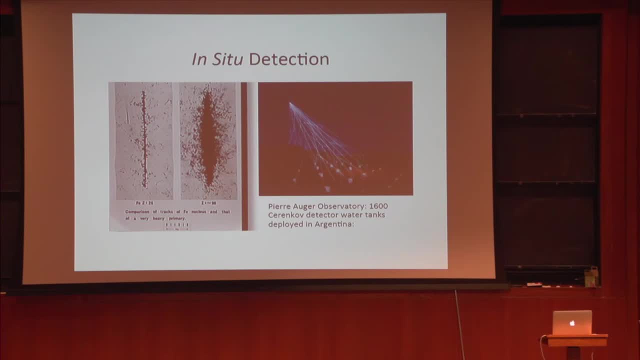 Pierre Auger observatory, which is 1600 Cherenkov detectors in the form of water tanks. and then It's in Argentina. a high energy cosmic ray comes in, it breaks up in the atmosphere, creates an air shower and the coincident detection of the cascade of particles from 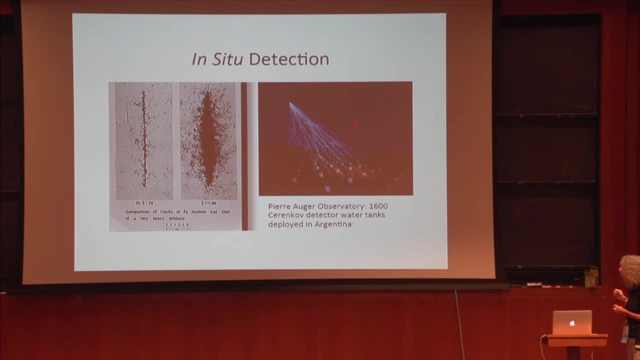 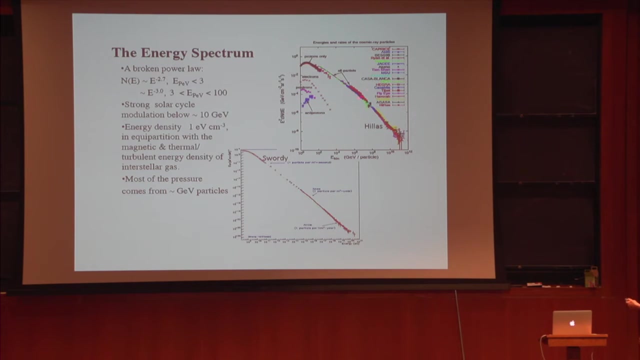 that air shower tells us something about the energy composition and direction of that original cosmic ray particle. But because we've never studied matter of the highest energy at the highest energies that we detect cosmic rays at, it's all a little bit speculative. Okay, so putting all that together, what is the energy spectrum at the Earth? 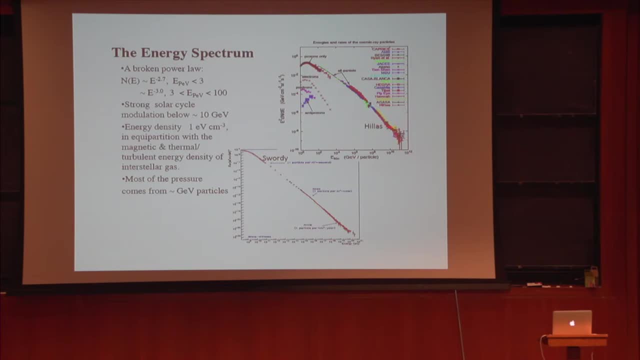 So here are two views of it. I'd like to show this one, because it not only has a tremendous amount of information on it, but it shows you the huge number of diversity of experiments that have gone into reconstructing this spectrum. Okay, So it's what we call a compensated spectrum multiplied by E squared. 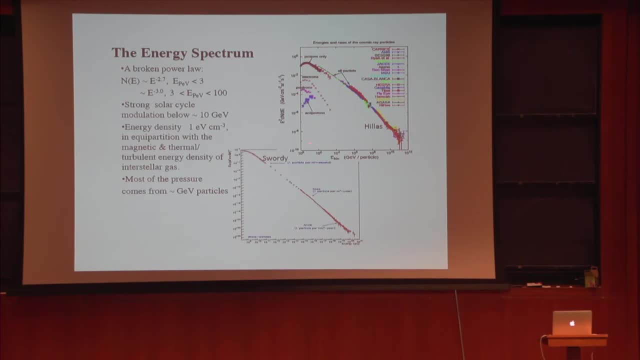 This is the energy in GeV per particle going up from 1 to 10 to the 12th, and you can see that the spectrum is basically a broken power law. Here are the slopes and the breaks. the spectrum below about 10 GeV is a little bit uncertain. 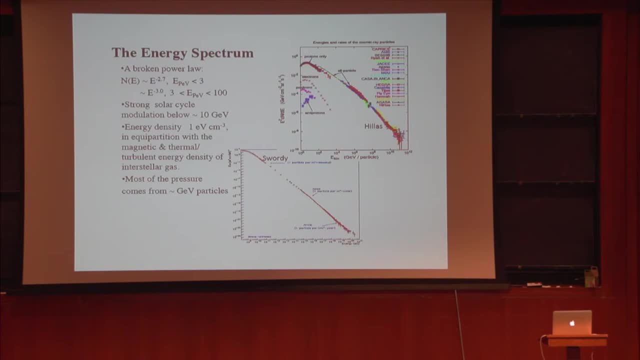 because of strong modulation by the solar wind. so there's a big solar cycle effect for low energy cosmic rays. If we extrapolate what we see at the Earth to the interstellar medium, we see that the energy density represented by the spectrum is about 1 EV per cubic centimeter and that 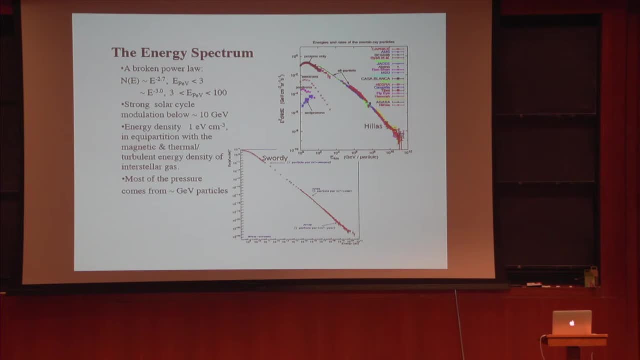 puts it into rough aqua partition with the magnetic, thermal and turbulent energy of interstellar gas, And an important question is whether that holds up in all galaxies. We recently have evidence that it doesn't. So these very high energy particles are fascinating but they don't really do much from an energy. 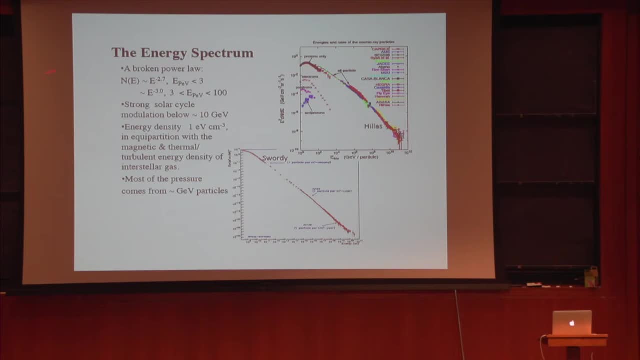 point of view. Most of the pressure and energy density in cosmic rays comes from particles with huge GeV, And if we look at this sort of cleaned up spectrum down below, we can see what the flux of cosmic rays of the Earth actually is. 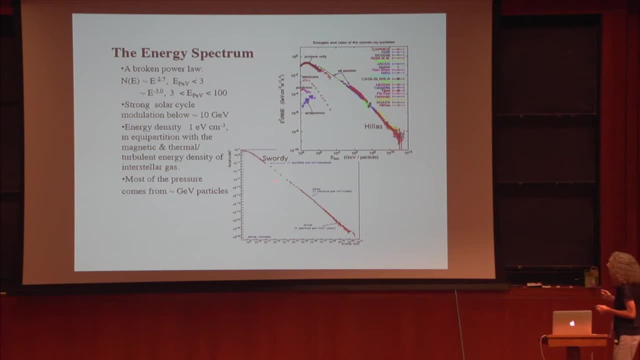 So here at low energies, particle per square meter per second. Here at the knee, one particle per square meter per year, And here at the so-called ankle- so these features are named after parts of the leg- there's one particle per square kilometer per year. 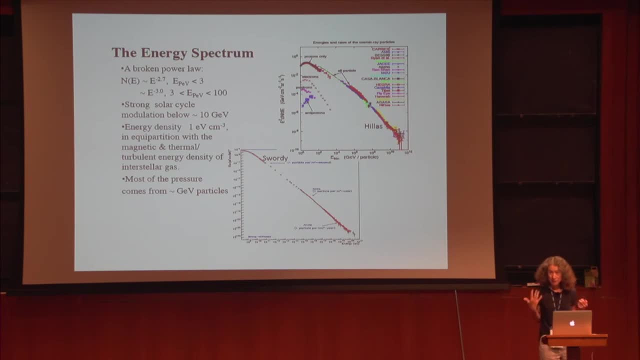 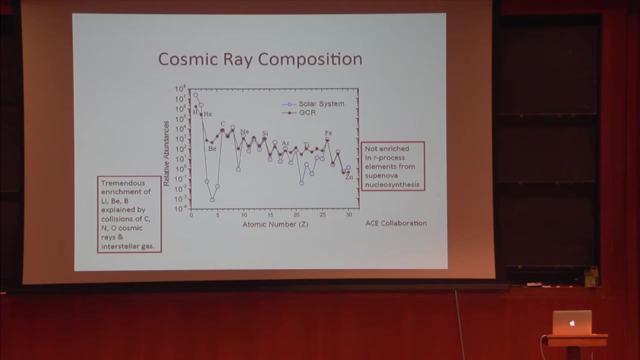 So detecting the highest energy cosmic rays and accumulating statistics on them is a huge challenge. Okay, here's the composition of cosmic rays as seen at the Earth compared to solar system composition. So what do we see? Well, we see a certain amount of similarity, but we also see some big differences. 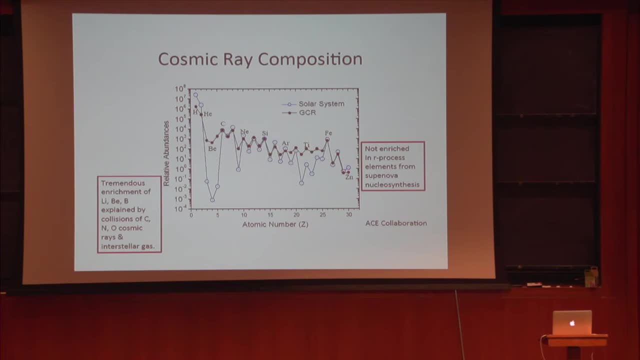 And the biggest difference that we see is that cosmic rays are tremendously enriched in lithium, beryllium and boron. Now, these are not products of stellar nucleosynthesis, Because they're fused. They're fused and destroyed at too low a temperature. 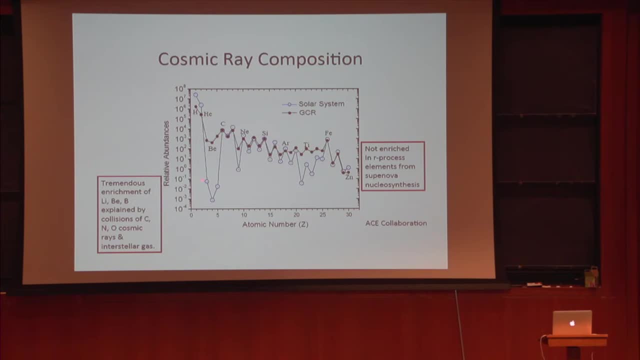 The most straightforward explanation of why there's the light element abundance is so high is that carbon nitrogen and oxygen cosmic ray nuclei are shattered by collisions with interstellar particles. So, assuming that the initial abundance is essentially zero, we can tell how much matter. 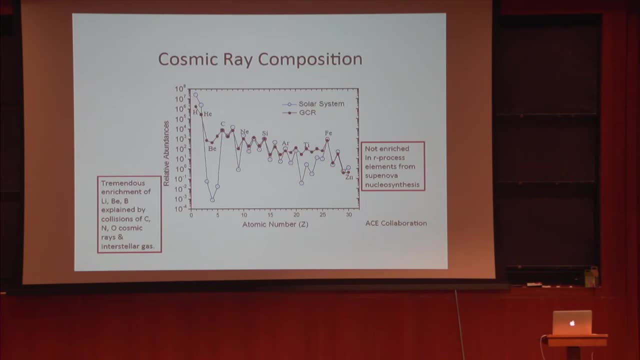 cosmic rays have passed through between the two, Okay, Between the time they were accelerated and the way to Earth. Now, something of a surprise was that the cosmic rays are really not enriched in the R process elements associated with supernova nucleosynthesis, And the expectation was that they would be. but they're not. 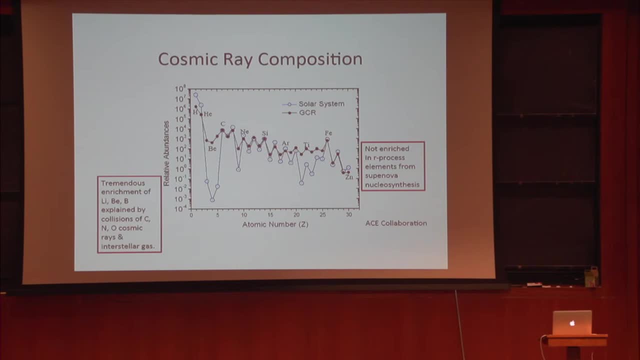 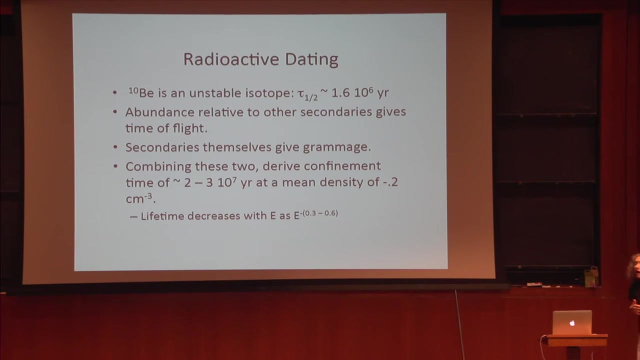 And this is strong evidence that cosmic rays are not directly supernova ejecta. So in the most literal sense they're not. But in a more extended sense we'll see that they were most likely right. So we can go a little further with reconstructing cosmic ray history by radioactive dating. 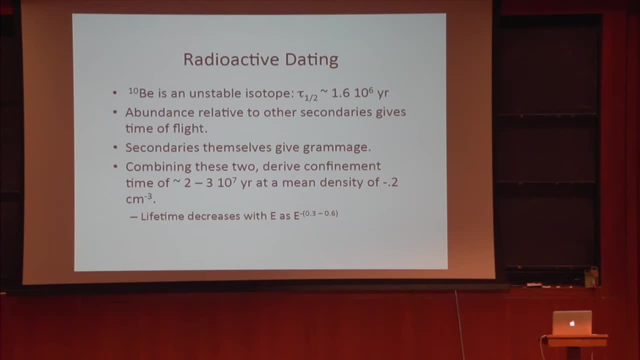 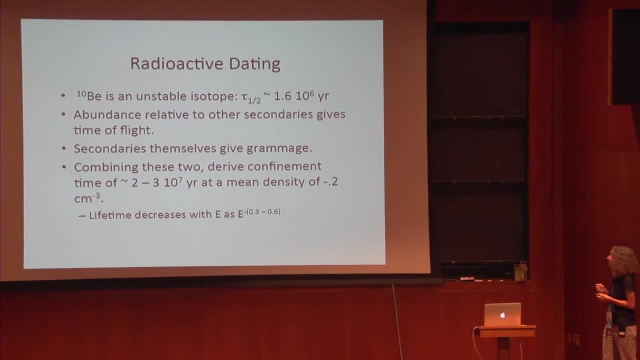 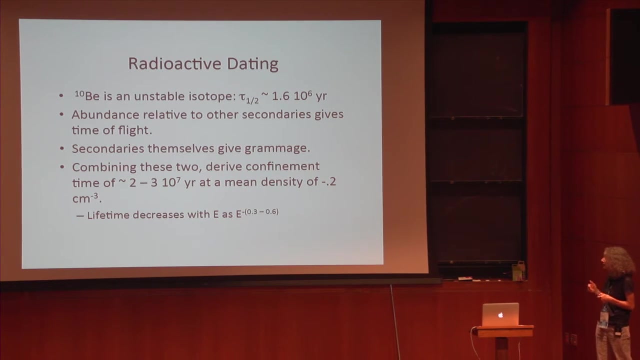 So there's this unstable isotope, beryllium-10,, with a long half life, 1.6 million years, And by measuring its abundance relative to the other secondary, we get some data. we can tell not only how much matter cosmic rays have passed. 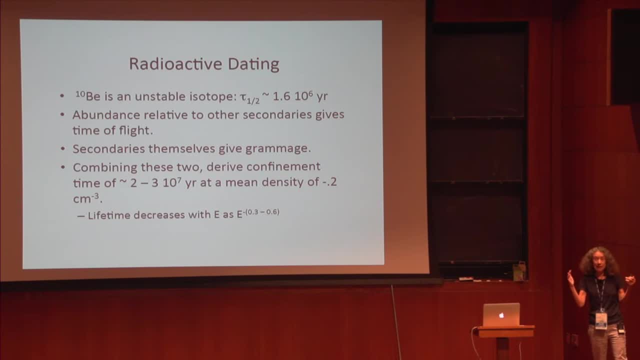 through on the way to Earth, but how long it's actually been since they were accelerated, And that implies that cosmic rays are confined in the galaxy for somewhere between 20 and 30 million years, And the average density of the confinement volume is about 0.2. 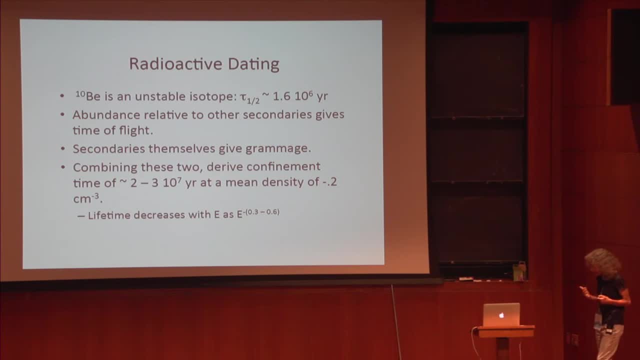 per cubic centimeter And that's about 1 fifth of the density average density in the disk of the galaxy. But as we'll see, that's OK. The lifetime is not constant with energy. It actually decreases as a small fractional power of energy. 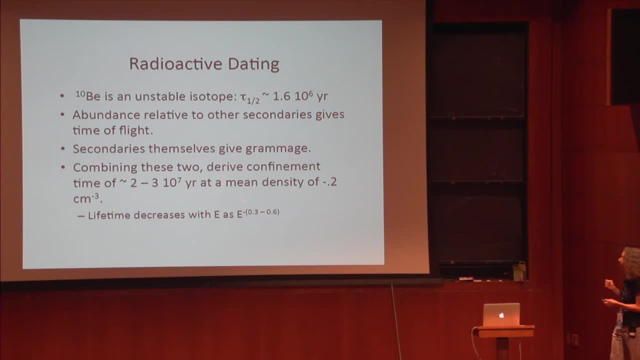 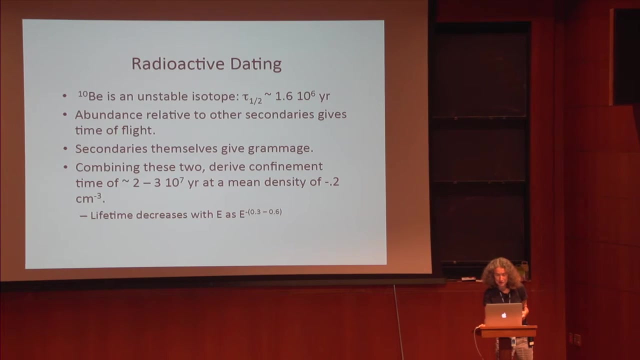 So the higher energy cosmic rays, but this is only measured up to a few hundred close to t, t To a TeV, so not the highest energy cosmic rays. the higher energy cosmic rays are not confined for as long as the lower energy ones. 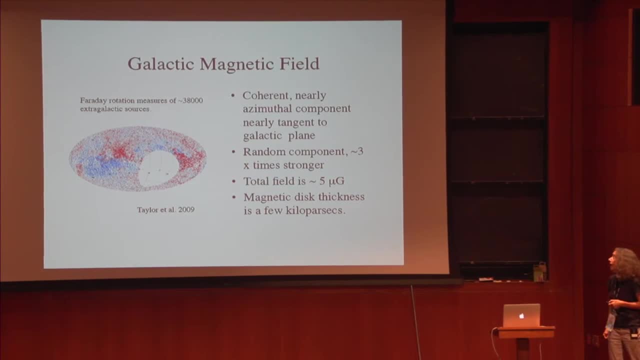 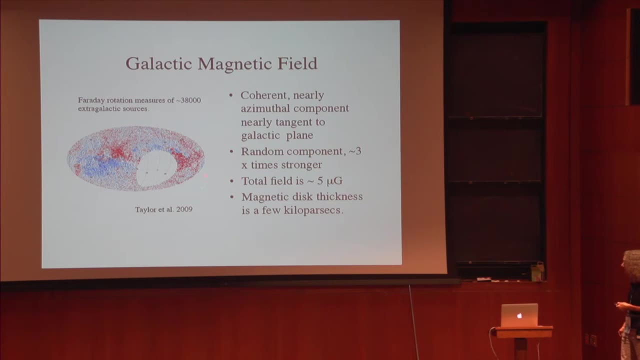 OK, so you can't talk about cosmic rays without talking about galactic magnetic fields. Here is the galactic magnetic field revealed through Faraday rotation of extragalactic background sources. So for those of you who are not astronomers, you should really take. 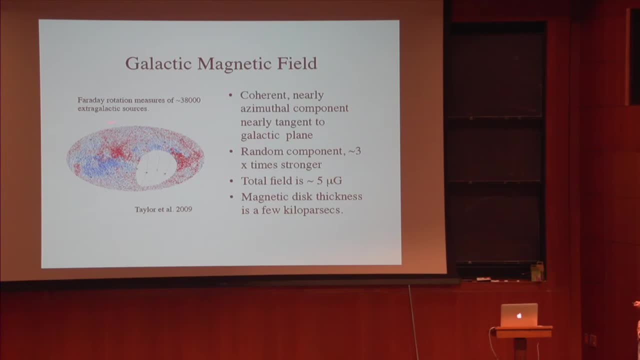 this in. There are 38,000 extragalactic sources represented on this plot. Blue and red represent positively and negatively directed fields along the line of sight with respect to the Earth. So you can see that there's a lot of long-range order. but 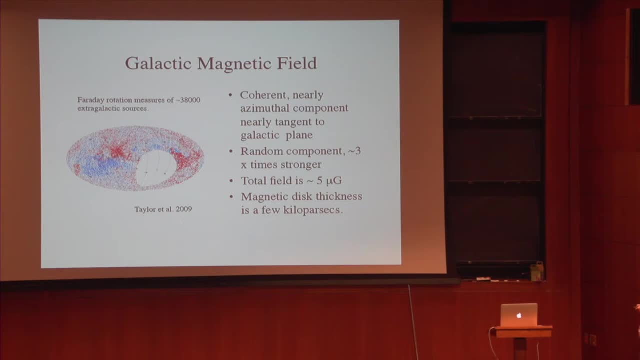 there's also a certain amount of disorder here. Putting this and other forms of evidence together, we can conclude that there's a coherent component to the galactic magnetic field. It tends to be azimuthal, It's nearly parallel to the galactic plane, but there's 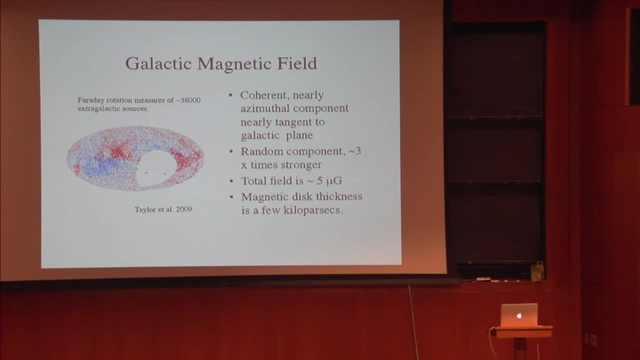 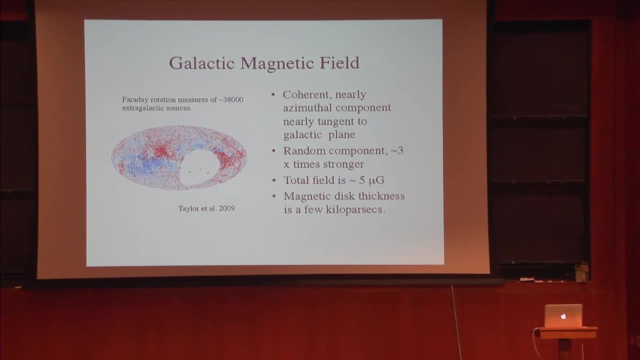 also a random component which is a few times stronger. The total field is about 5 microgauss and the thickness of the magnetic disk is a few kiloparsecs. And that is thicker than the gas, the dense gas, in the disk. 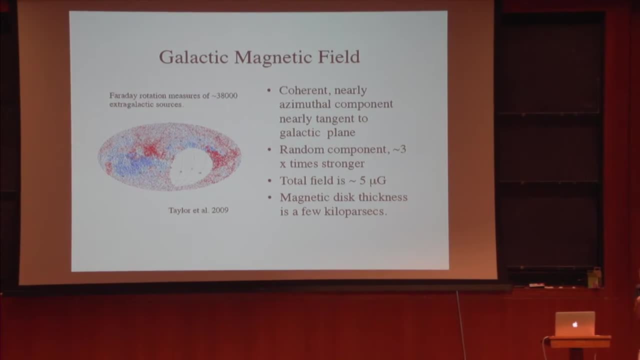 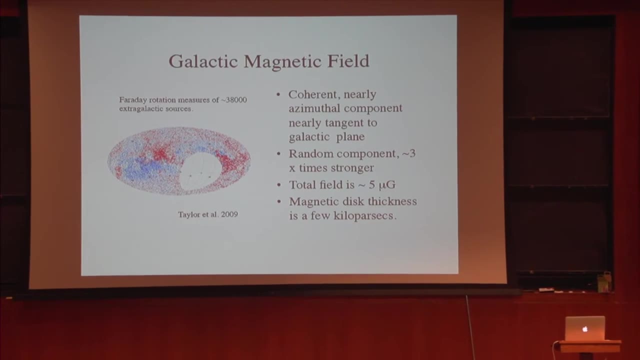 And so that's the problem. That's how we can reconcile the fairly low average density that cosmic rays live in. They occupy a thick magnetized disk. They spend some of their time out of the galactic plane- actually most of their time out of the galactic plane. but 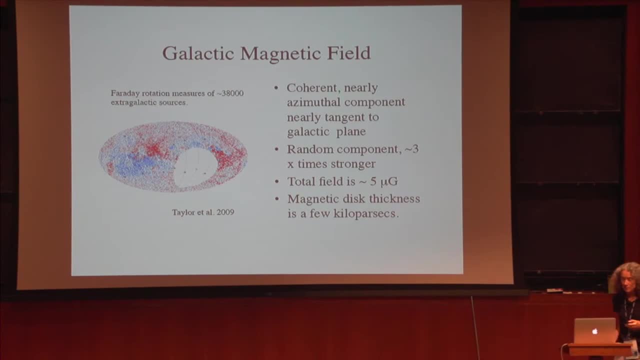 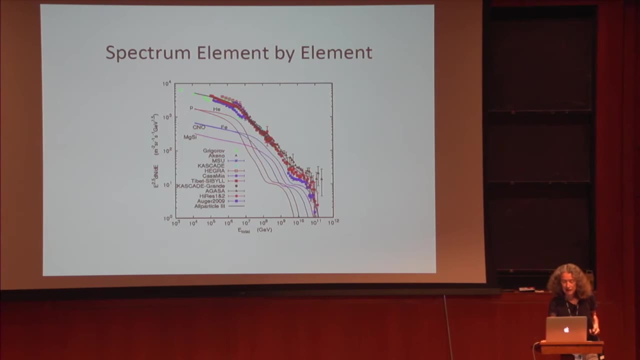 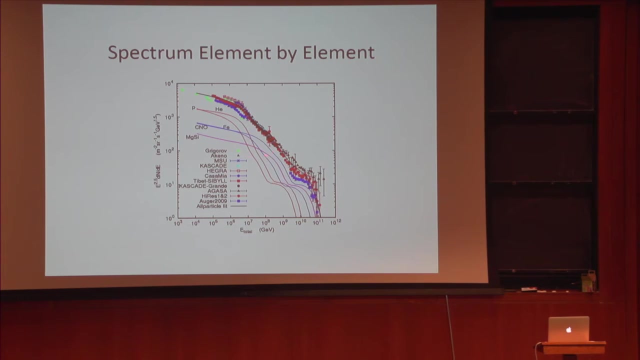 they keep whizzing through and showing up in the neighborhood of the sun. Is this all reasonably clear, OK, So if we break down a little bit, If we break down the spectrum element by element, we can see things actually get really complicated. 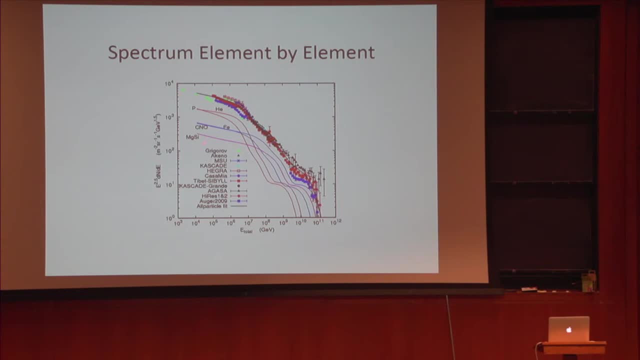 And I'm not even going to attempt to explain this, but I thought that you should know about it. So the proton spectrum is not the same as the helium spectrum, which is not the same as the iron spectrum or the CNO spectrum. They have different features, particularly at the highest. 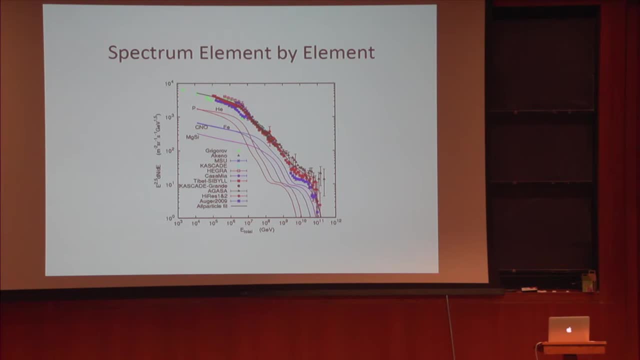 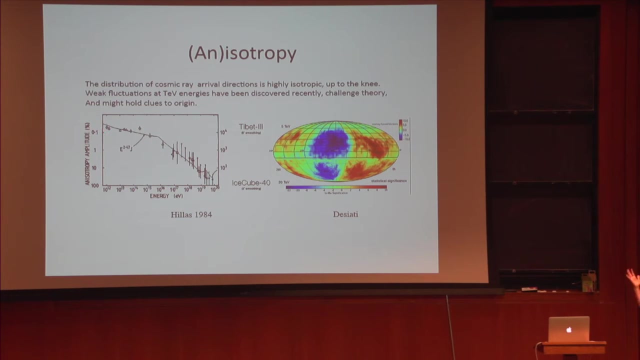 energies, And this probably represents some joint effects of acceleration and propagation which we can say a little bit more about later if we have time. Cosmic rays arrive at the Earth virtually isotropically the same in all directions. This is the anisotropy as a function of energy. 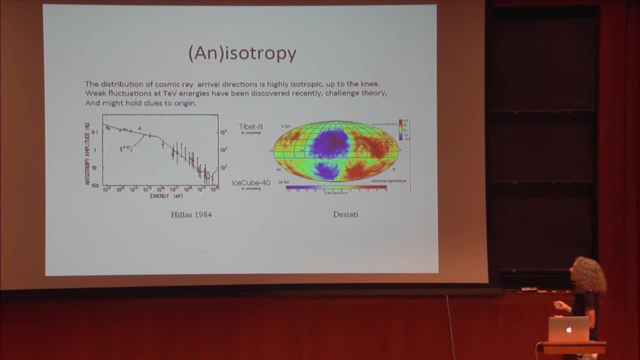 And you can see that at- since this is EV now, not GEV, you can see that Up to a TEV they're isotropic to better than a tenth of a percent. And then, as we go to the highest energy cosmic rays, the 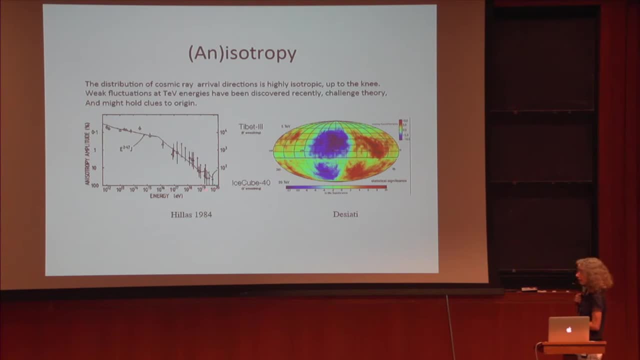 anisotropy becomes quite strong. So this goes all the way to 10, to the 20th EV. Recently, in the last decade or so, some kind of puzzling anisotropies have been discovered in cosmic rays. So this is at the TEV and above level. 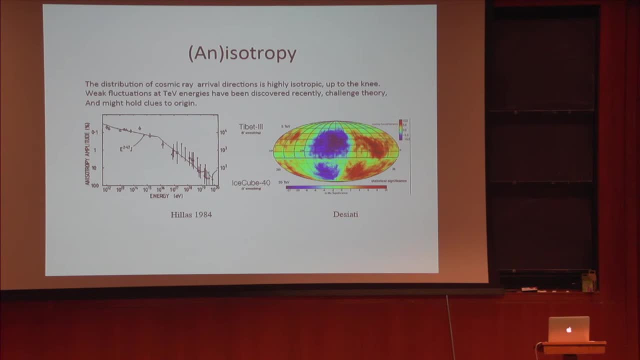 They're very small. They're well, they're hundredths of a percent. It's a little bit like the fluctuations in the CMB. They're very small amplitude but they're very important And if we knew how to interpret this anisotropy, we would 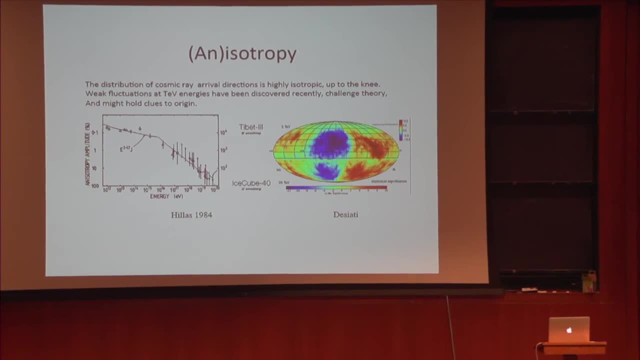 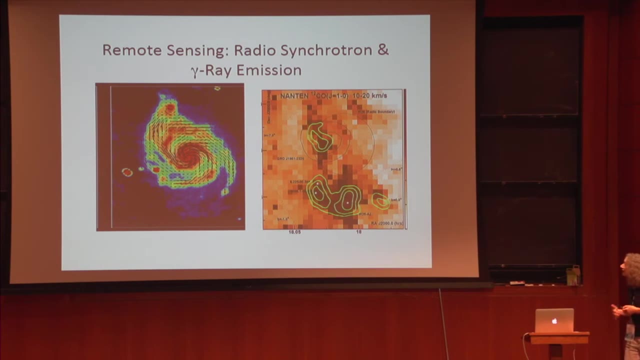 probably learn something about how cosmic rays propagate and maybe even what their sources are. OK, so cosmic rays that are not in the solar neighborhood. So for a long time we've been able to observe synchrotron radiation, a non-thermal radio continuum, from external. 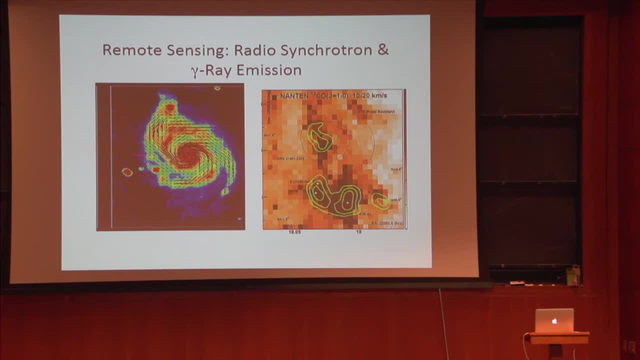 galaxies And this is an image of the spiral galaxy M51.. The colors represent brightness And the little black line segments represent the orientation of the plane of the sky, magnetic field as revealed by the polarization of synchrotron radiation, And we can see. 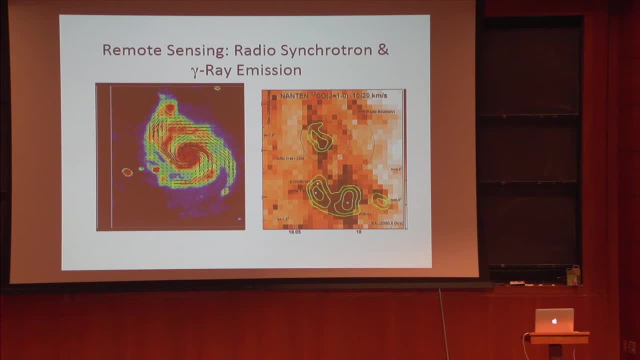 We can see that the field sort of follows a spiral-like pattern, but there are certainly patches of disorder. That tells us what the electrons are doing, And here in our own galaxy is an image of gamma ray emission superimposed on radial brightness contours from the. 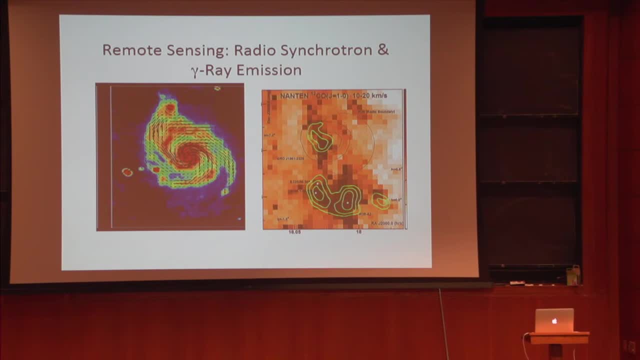 carbon monoxide molecule And what this tells us is that dense molecular clouds are copious emitters of gamma rays And they're not interactions. They're not Federation advance images. That probably means that the cosmic radiation that they're bathed in, those cosmic rays are interacting with that. 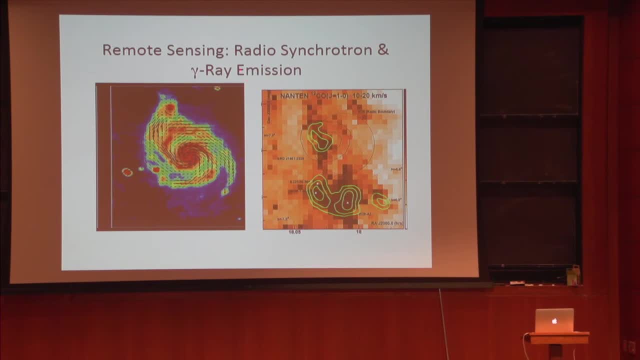 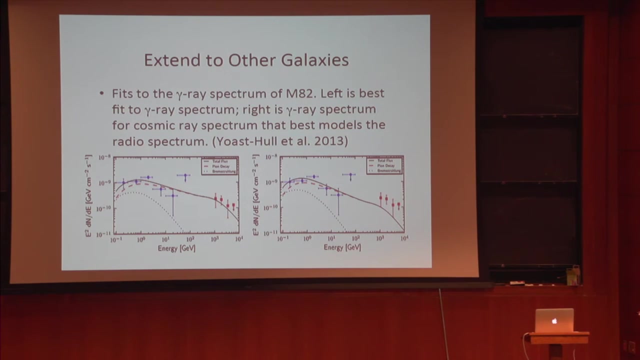 dense gas making charged and neutral pions, and the charged pions decay to electrons and positrons and the uncharged pions produce gamma rays. So we can get pretty quantitative in fitting gamma ray and radio spectra of other galaxies And here's one example: the Starburst Galaxy M82.. 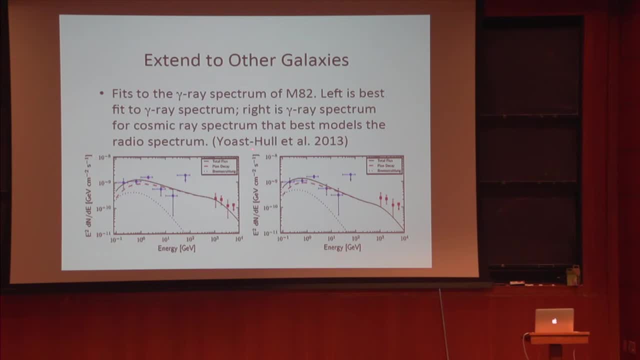 This is work by a recent PhD student, Tova Joost-Hall, And the, So the data is the same in both these images. The blue points are from Fermi, The red points are from Hess. It goes up to about 10 TeV. 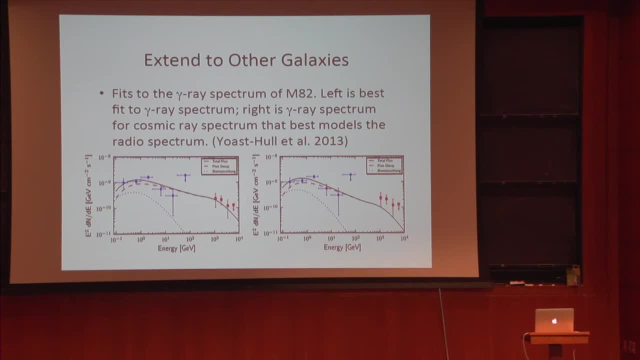 And the solid lines are two fits to the spectrum. The fit on the left is the best fit to the gamma ray spectrum And the fit on the right is derived from the cosmic ray distribution that's best fit to the gamma ray spectrum. The best fit's the synchrotron spectrum. 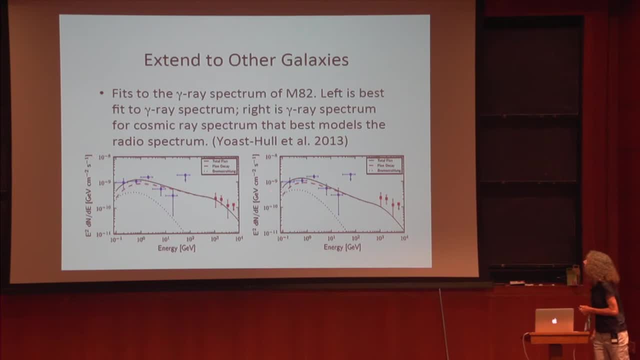 So we have gamma ray and synchrotron spectra from both from this galaxy, And you can get pretty good fits. Now what's astounding to me is that this is done with Milky Way-like assumptions. We assume that about 10% of supernova energy goes into 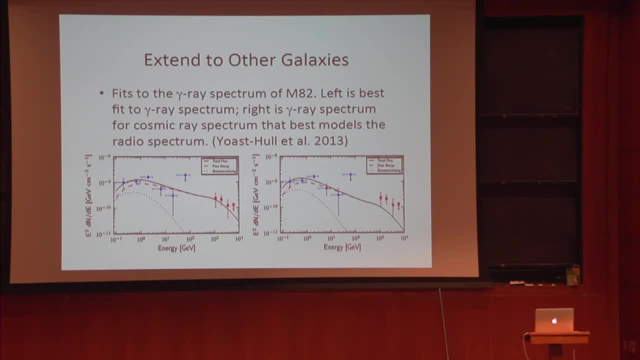 cosmic rays, that there are about 50 times as many protons as electrons just as there are on Earth, That they propagate in very similar ways And it's possible to get a very good fit to the spectrum with these very simple assumptions. 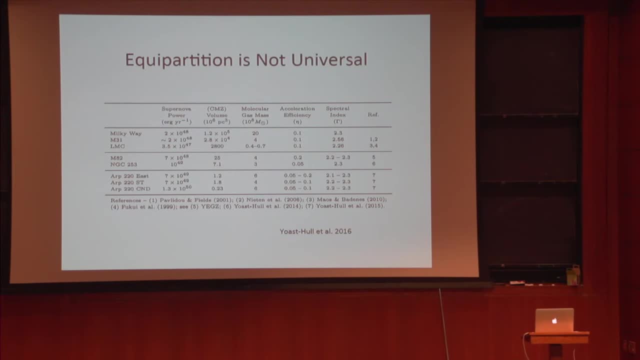 So by comparing gamma ray and radio emission from many galaxies, it's possible to test this assumption of equipartition that holds so well in the Milky Way. So here are several different galaxies, so the Milky Way M31, which is very similar to our galaxy, the Large Magellanic. Cloud nearby dwarf, the Starburst Galaxy, M82, and NGC 253.. So these are galaxies with much higher star formation rates than the Milky Way. And then here, ARP 220, it's a galaxy merger that we're catching. 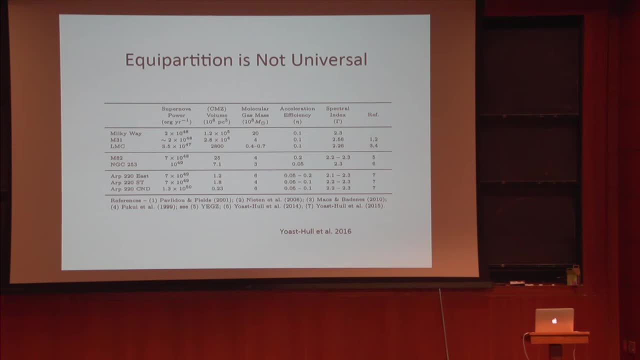 So there are two nuclei that are orbiting each other And very dense, very high star formation rate, et cetera, And here are some comparisons for models that we've tried to fit. I put the wrong figure in here, So I actually have a figure. 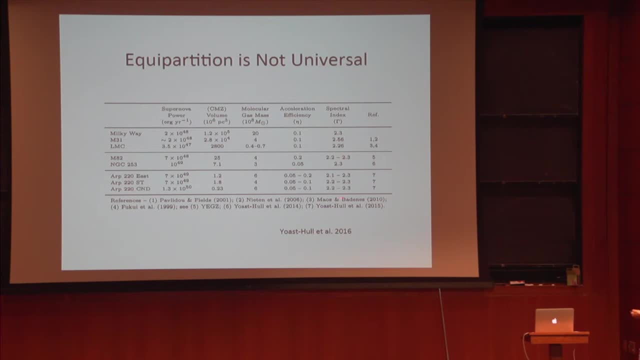 This is really embarrassing. I actually have a figure that shows that the cosmic rays are not keeping up, And when I The notes online will have to show this figure. Sorry, But I'll tell you in words that, although equipartition holds in, 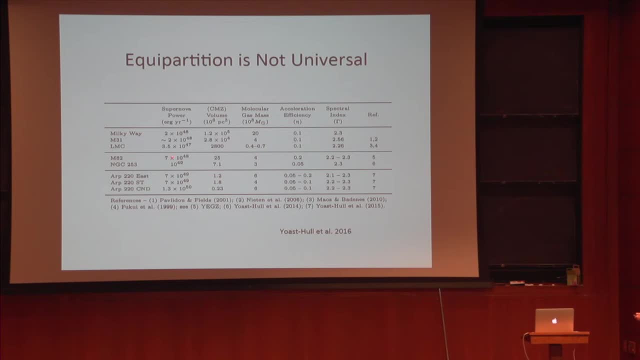 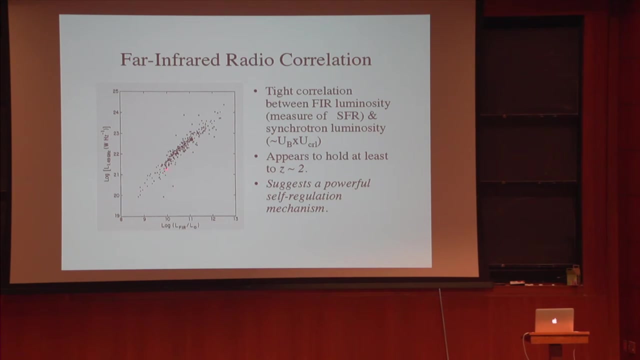 the Milky Way. the cosmic rays drop further and further behind as we go to galaxies, with higher and higher star formation rates, And this is probably because the losses are very high. OK, Then, at a less detailed level, there's this far infrared radio. 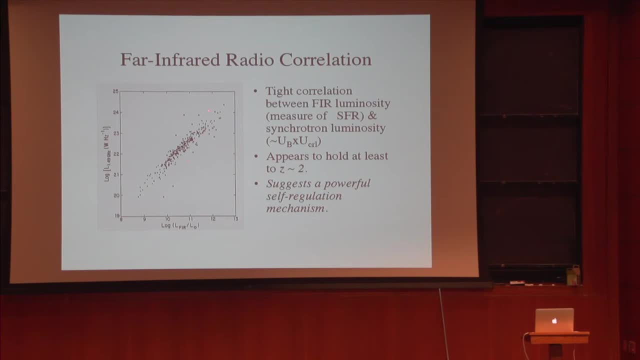 correlation. So there are many, many galaxies represented here. They range over several orders of magnitude in far infrared luminosity and synchrotron luminosity, And yet there's quite a tight correlation between the two. The far infrared luminosity is a measure of the star formation. 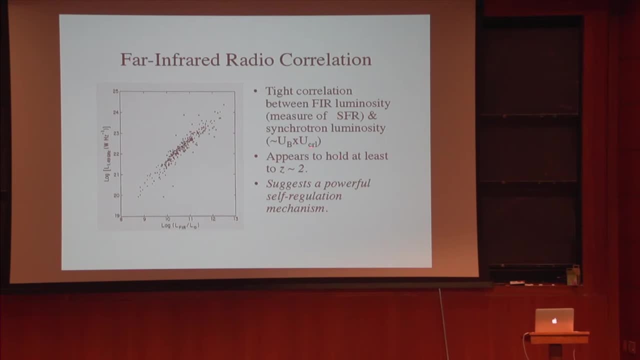 rate And the synchrotron luminosity is basically the product of the magnetic and cosmic ray energy densities And this holds back out to a redshift of about two, so when the universe was just a few hundred thousand years old, And this really suggests that there's 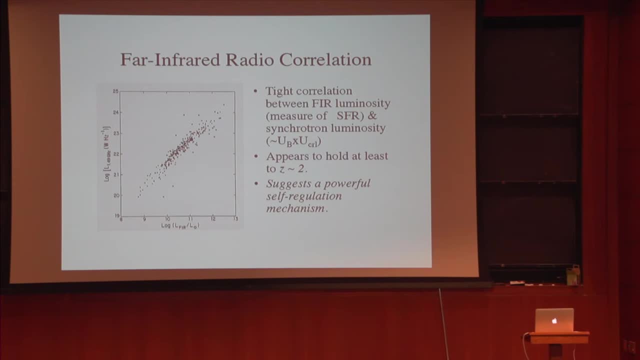 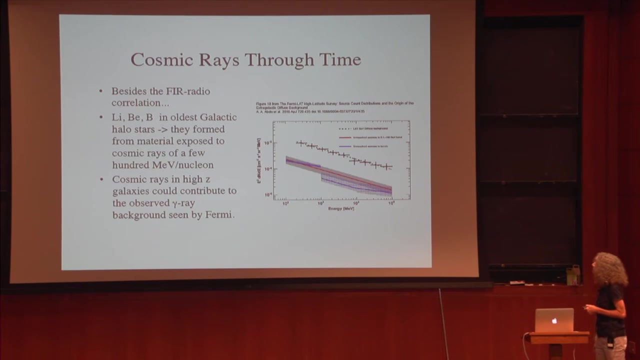 a powerful self-regulation mechanism that controls that links star formation, magnetic field evolution and cosmic ray acceleration and propagation. We can go back even further in time In our own galaxy. there are light elements that are detected in the atmospheres of the oldest. 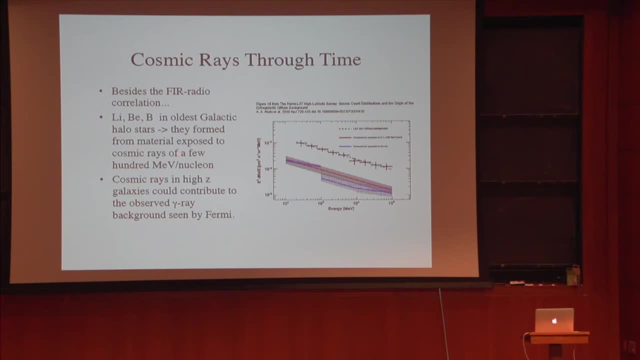 halo stars, And the most straightforward explanation for those light elements is that those stars formed. the oldest stars in our galaxy, formed from material that had been irradiated by cosmic rays, Not necessarily very energetic, but up to a few hundred MeV per nucleon. 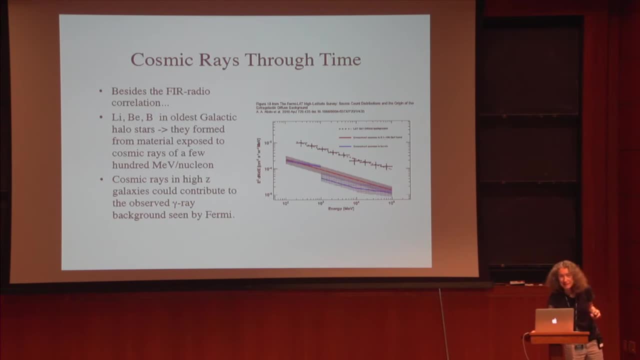 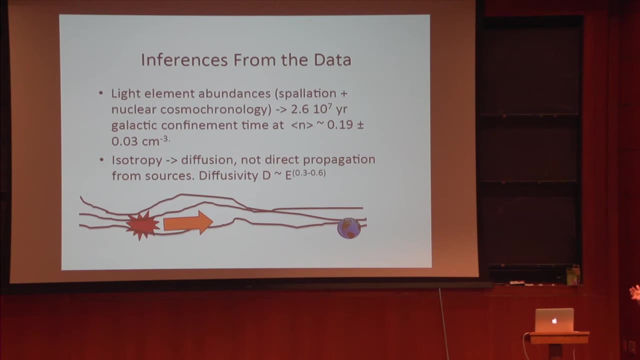 So cosmic rays and magnetic fields in some form have been around for a long time. OK, So let's try to draw all these observations together and come up with a smaller set of things that we can explain. So, from the light element abundances. 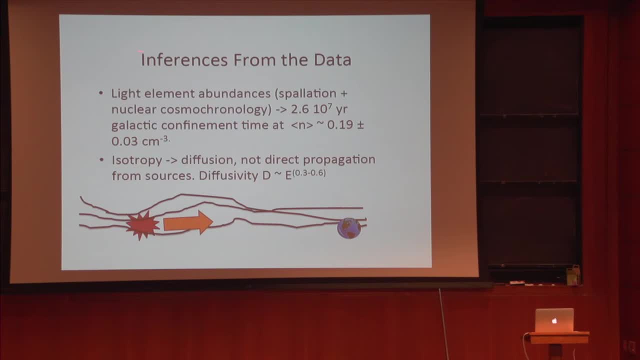 and the nuclear cosmocronology. the radioactive dating cosmic rays are confined in the galaxy for about 26 million years And the mean density that they propagate through is about 0.2.. And there is a reason for that: Because they arrive at the Earth nearly isotropically. 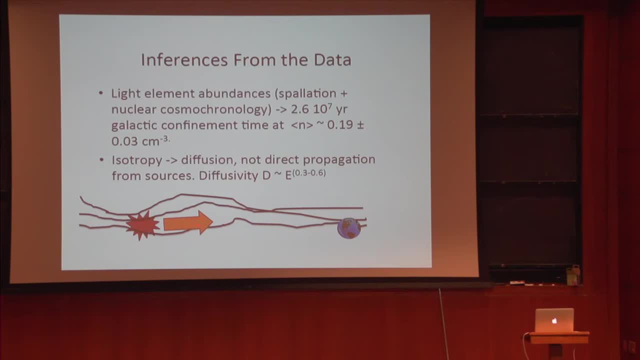 and because they clearly rattle around in the galaxy for a long time, they must propagate diffusively rather than directly. So if here's a cosmic ray source and here's the Earth, the cosmic rays don't just kind of arrive in a blast down the magnetic field lines. just from the source to the Earth. That's not what we see: isotropic, very old particles. We can also say that similar processes occur in other galaxies: The radio and synchrotron- sorry, the synchrotron and gamma ray emission from other galaxies. 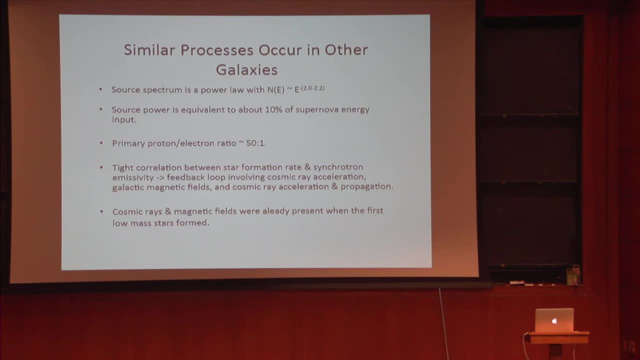 is well represented, if we assume that there's about 10% of supernova energy creates cosmic rays with a power spectrum of about e to the minus 2, which is not quite as steep as the observed spectrum. There are aging processes like escape and energy loss that steepen the spectrum a little. 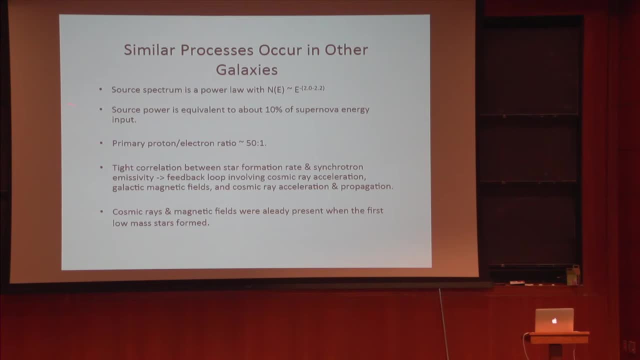 bit That the proton to electron ratio is about 50 to 1 in the source. There's this tight correlation between the star formation rate, the synchrotron emissivity and the So magnetic field, Magnetic fields and cosmic ray energy densities, suggesting that there's some sort of feedback. 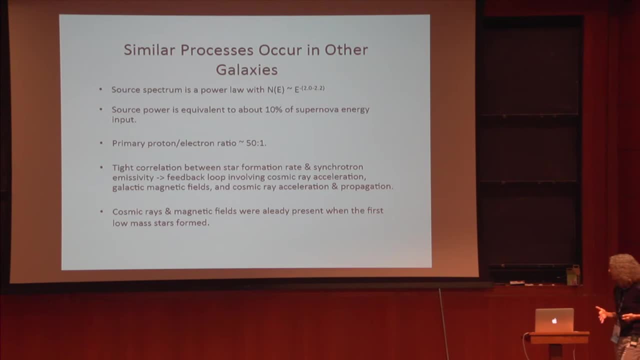 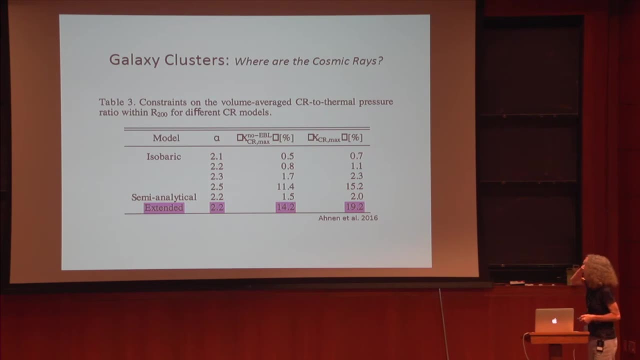 and it's been going on for a long time. Cosmic rays and magnetic fields were already present when the first low mass stars formed. Let's just say a word about galaxy clusters. So galaxy clusters are huge, massive aggregates of thousands of galaxies. They often have one or more active galaxies. 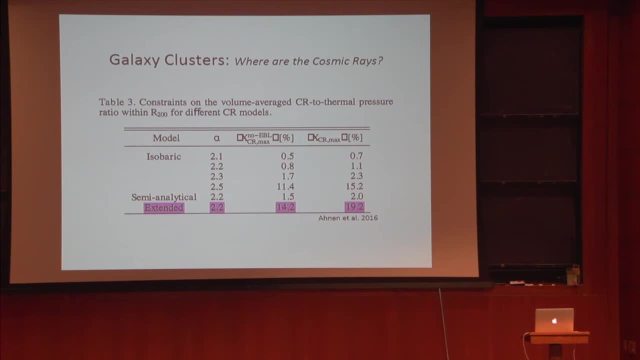 And the expectation was that galaxy clusters would be gamma ray emitters, But the gamma rays have really not been seen. When you, If you, look in the core of the cluster and you subtract gamma ray emission from point sources, the ratio of cosmic ray pressure to thermal pressure seems to be tiny. 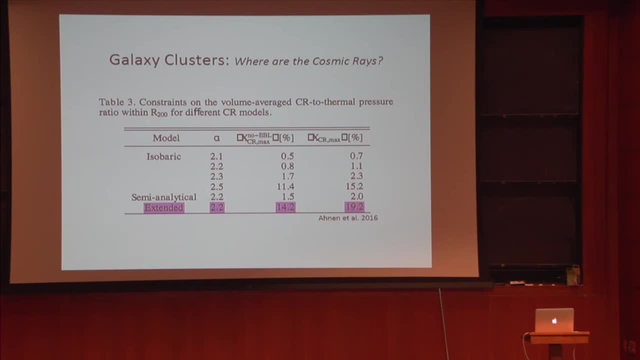 If you assume, on the other hand, that cosmic rays are produced in the solar system. the cosmic rays are produced in the solar system, And that's not true. If you assume that things go in the core of a cluster, where the active galaxy and the 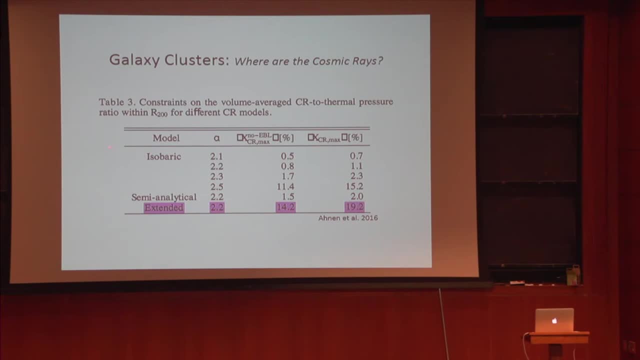 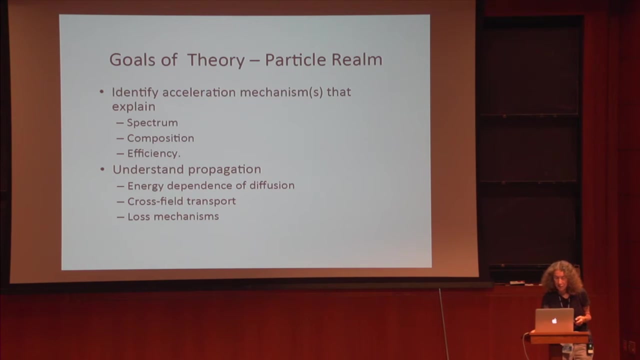 other massive galaxies are, and that they then propagate, disperse throughout the cluster. you come out with sort of larger averages and that fits the data better. So there are mysteries about cosmic ray propagation in galaxy clusters that are not well understood. Okay, So what would we like to do with all this? 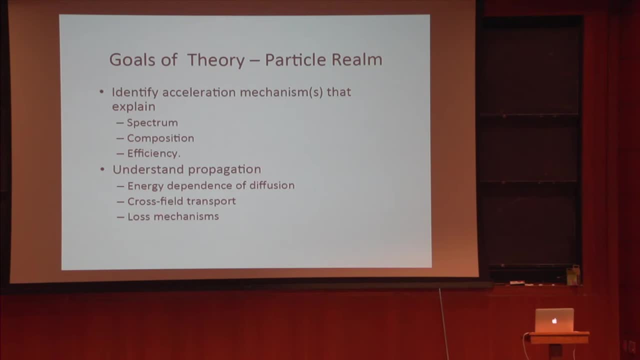 Yeah, Yeah, Yeah. So, from the particle point of view, we'd like to identify how cosmic rays are accelerated, We'd like to explain the spectrum, the composition and the efficiency of acceleration, And we'd like to understand how they propagate. what accounts for the energy dependence of? 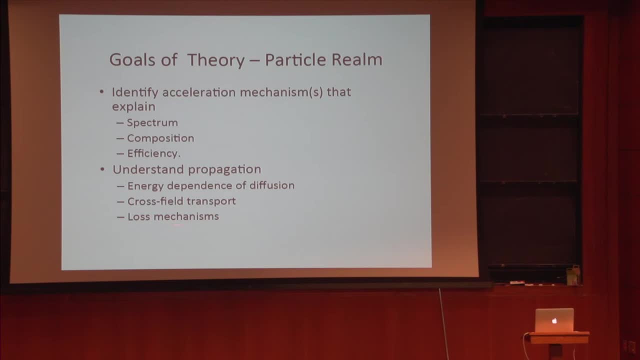 diffusion, whether they ever cross magnetic field lines and how they lose their energy. And then, from a collective point of view, we'd like to understand how they interact and modify the medium that they propagate in. They provide some hydrostatic support in galaxies, maybe a little bit in galaxy clusters. 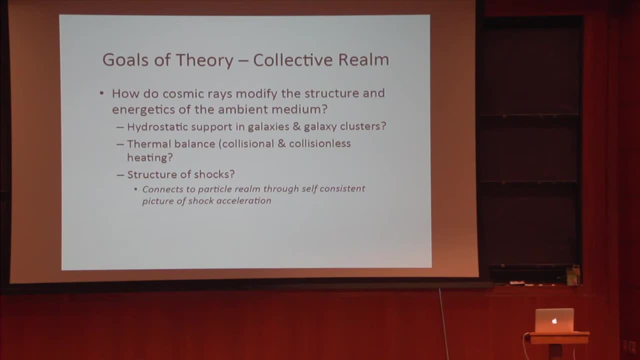 They heat the gas, Both collisionally and collisionlessly- although I don't think we'll get into that today- And they modify the structure of shocks. And this in particular kind of connects the collective realm with the particle realm, Because developing a self-consistent picture of how cosmic rays are accelerated in shocks 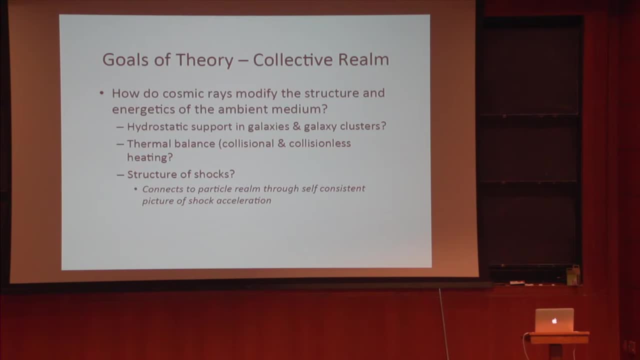 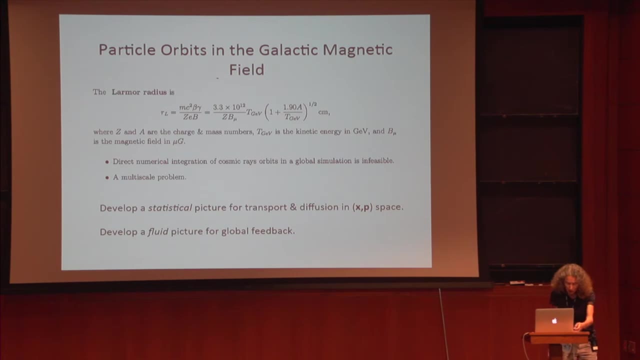 requires understanding also how cosmic rays modify shocks And, as we'll see, they can probably do that quite substantially. Okay, so any questions right now about this sort of whirlwind tour of properties? Yeah. Male Speaker 4. Female Speaker 2: Yeah, 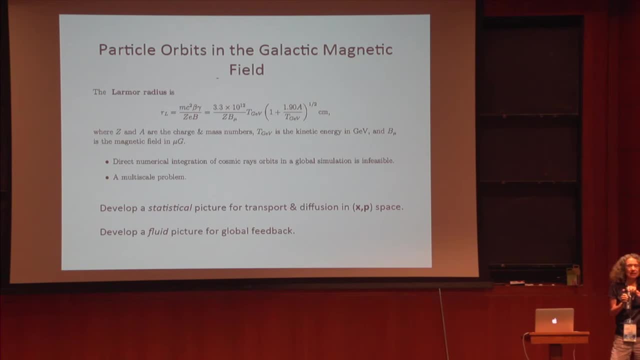 Male Speaker: 3. Yeah, So what does that say? So are you asking how that can be, how those two things are consistent, or what the implications are? Yeah, I'm not Sorry what? Yeah, so that's a good question. 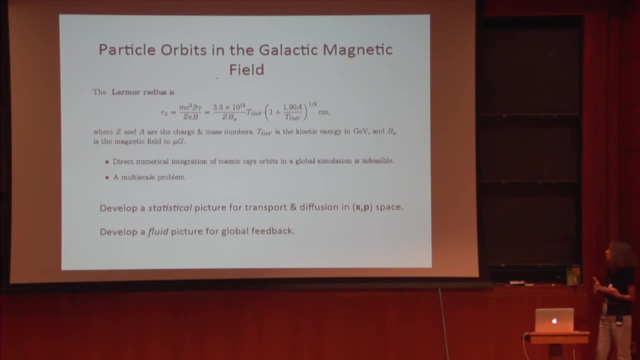 So let me write down a very simple equation for what determines the energy density in cosmic rays. So this is my. Is this visible? Good, Great, Okay, Okay, I don't know if I can do that with everything. Okay, So the rate of change of the cosmic ray number, density, is the source which is positive. 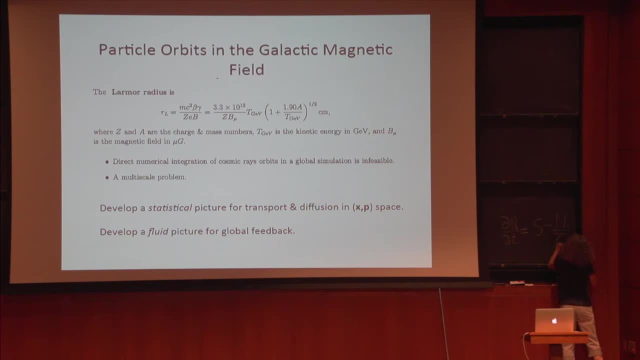 minus some type of loss, And I didn't get into what the losses are, but the most important sources of loss are direct collisions and some sort of advection, And so I'll memorize this and then we'll talk more about it. Yeah, 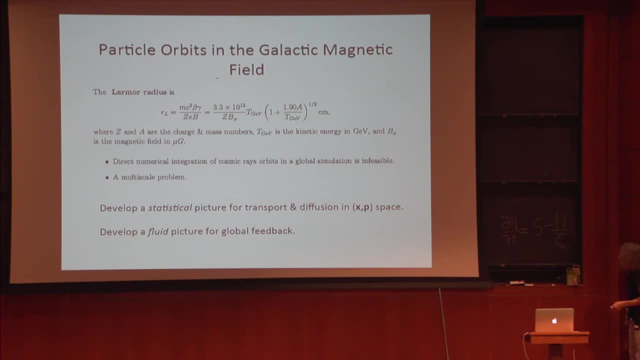 I think you might be more a fan of. In general, the most common source is the loss time, which is the nth. The Nth is the number that you can get from every direction of a galaxy, either in a galactic wind or through maybe just diffusive scattering. 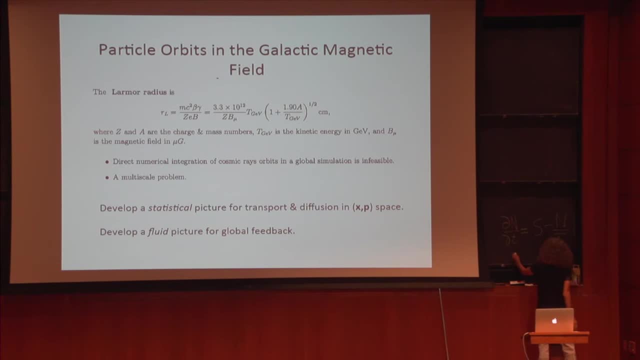 And so in a steady state, N is equal to the source times, the lost time. So what seems to be going on in objects like ARP 220 is that the lost time is very short. It can be as little as a few hundred years. 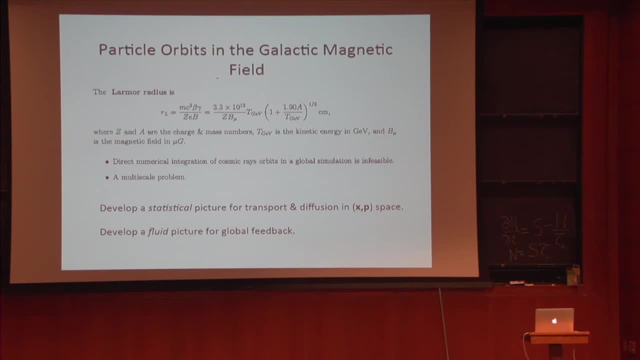 Whereas in the Milky Way it's more like tens of millions, And so the most common thing that we can do is to be able to find the loss time. it's more like tens of millions of years, even a hundred million years, and so even. 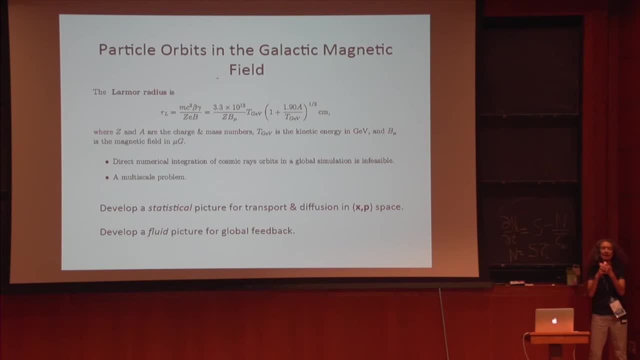 though. so even if the source is is copious, the cosmic rain number density or energy density will just be small. okay, now as for what this says about how cosmic rays would feed back on star formation, that is, that is such a big subject that we're only kind of scratching the surface because of the 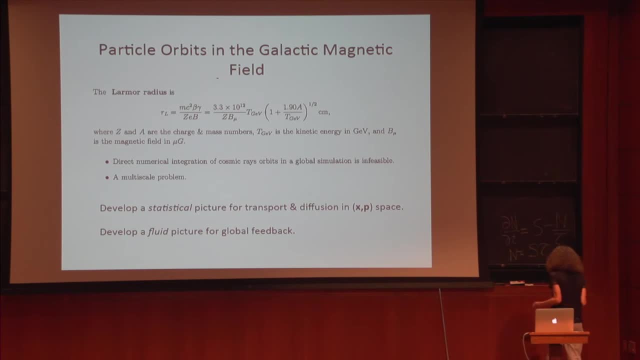 even though the cosmic ray energy density isn't keeping up with other forms of energy. in this object, the, the effect on chemistry is probably huge. so you know, there's this very kind of pedestrian chemical interaction: the, the ionization, the temperature of the molecular gas, they're all weird. so I 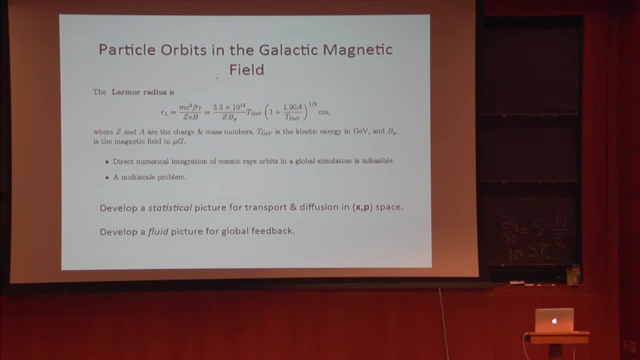 wish I could answer your question, but I really can't. it's a great question. any other questions? ok, let's go on and say a little bit about cosmic rays from a particle point of view and how they can cross magnetic field lines. so here's an expression for the Lama radius of cosmic. 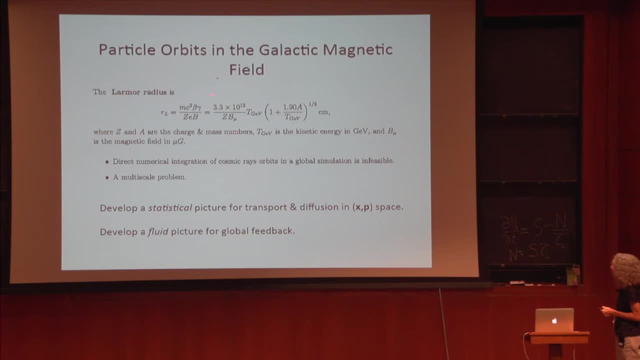 rays and t is kinetic energy in GEV And you can see that at a few GeV, in a magnetic field of a few microgauss, the Larmor orbit is well under an Au. Okay, so what does this mean? So, it means a couple things. 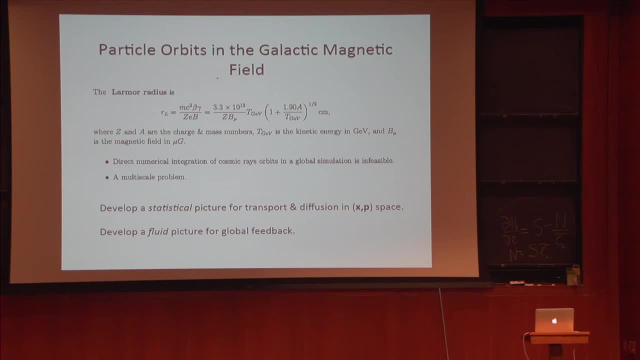 It means that direct numerical integration of cosmic ray orbits saying, well, okay, they're there, Let's just put them into our simulation and see what they do. It's just not feasible because the scales are so tiny, So it's really a multi-scale problem. 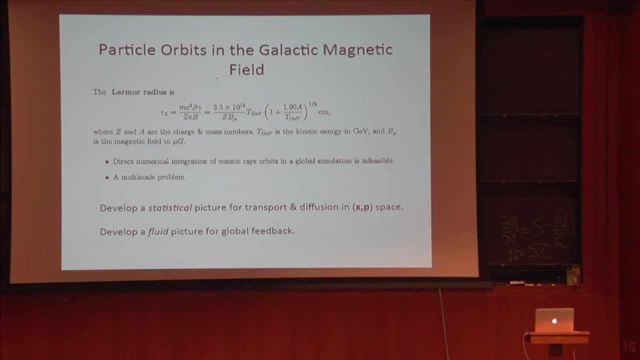 We can pick up a couple of other things from this. So if we go to the highest energy cosmic rays, so if we make this 10 to the 9, then this is about a kiloparsec, And so that means the Larmor radius is a kiloparsec in size. 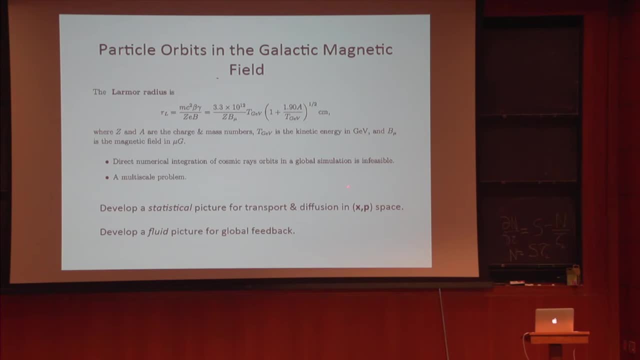 That starts getting hard to confine in the galactic magnetic field, And so we think that the highest energy cosmic rays are actually extra cosmic rays- Galactic. So what we need to do in order really to do anything with cosmic rays as an ensemble is 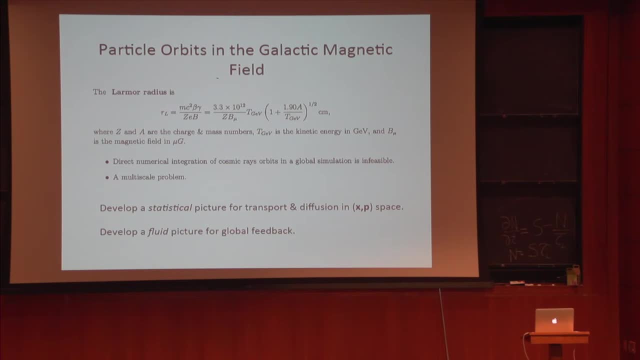 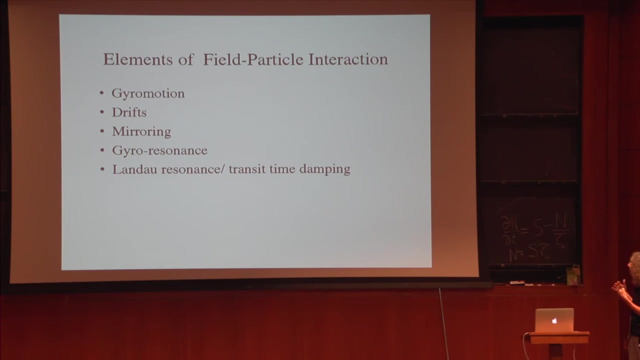 develop some sort of statistical picture for transport and diffusion in both position and momentum space And, as we said on the flow chart, this will allow us to develop kind of a fluid picture that we can use to study global feedback. Okay, So since we can't really integrate the gyro orbits, we can kind of break them up. 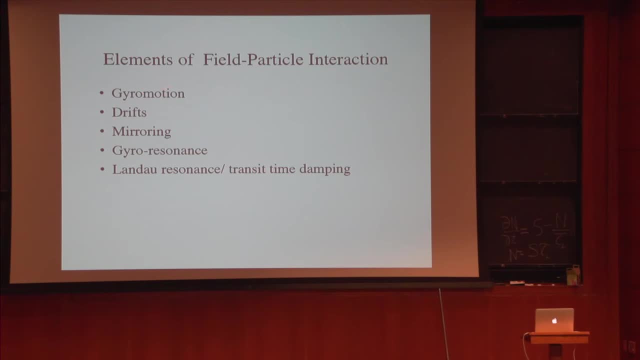 And I think this will be a review for most of you, but I just want to go through it quickly. The elements of the field particle interaction are first of all the gyro motion, then there are drifts, then there's mirroring, then there's gyro resonance and then there's the Landau. 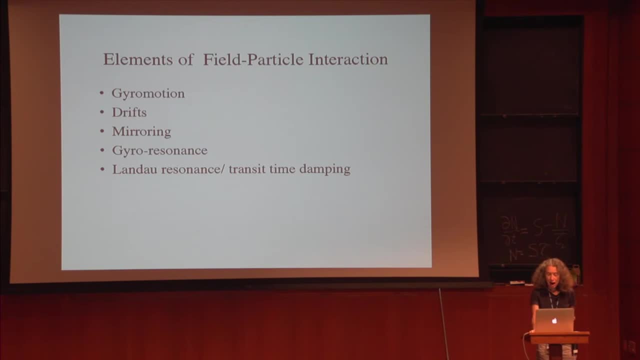 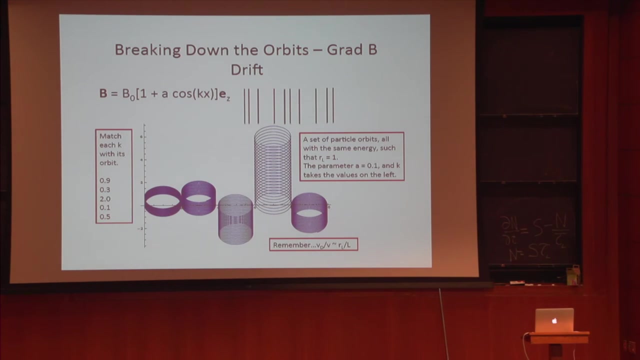 resonance and transit time, damping, And how many of these topics have we talked about? How many of these topics have been covered in previous lectures? One, two, three, four, five, One, two, three. Okay, Then you'll be able to answer this little problem. 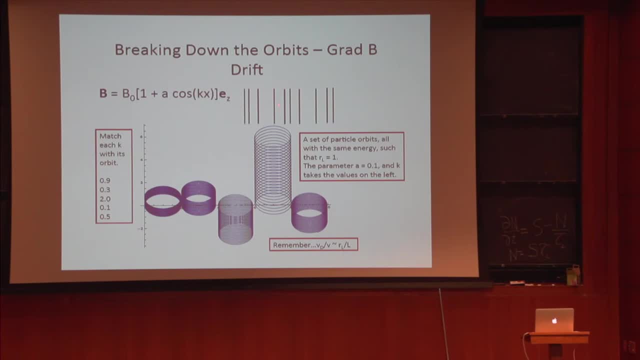 This is a review, So here's a very simple magnetic field. The field lines are straight, but the strength depends on position x. So here's a picture of that And here's a bunch of particle orbits. They all have the same energy. 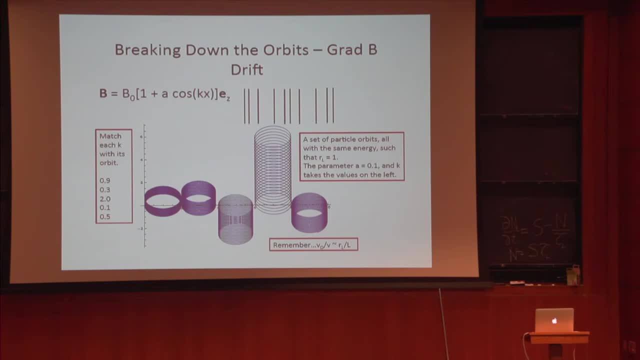 They're all the same size, but I've just spread out their origins here so you can tell them apart more easily. And this parameter, a, is set equal to 0.1.. This is the x-axis, This is a y-axis And the k the wavelength of variation. here there are five different values that are represented. 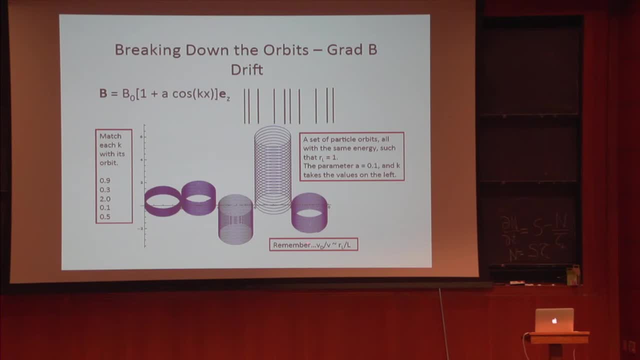 Okay. So first of all, why are these particles moving either up or down in y? That's a drift. Why is it in the y direction? So z is actually this way. It's just a little bit. there's kind of a perspective view here. 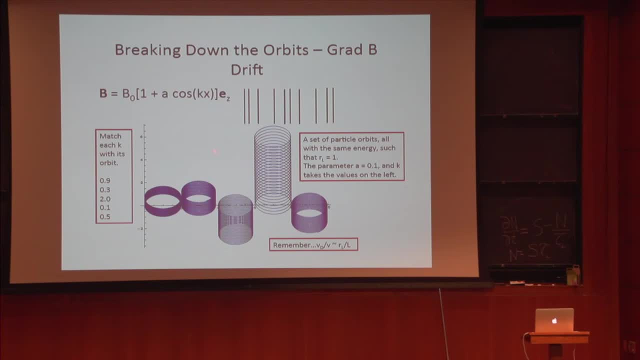 So, as we picture a particle gyrating in the xy plane, the strength of the field on this side of the orbit is different than it is on this side of the orbit. Now, remember that the acceleration is perpendicular to the motion. So a gradient in x will send it shooting up or down in y. 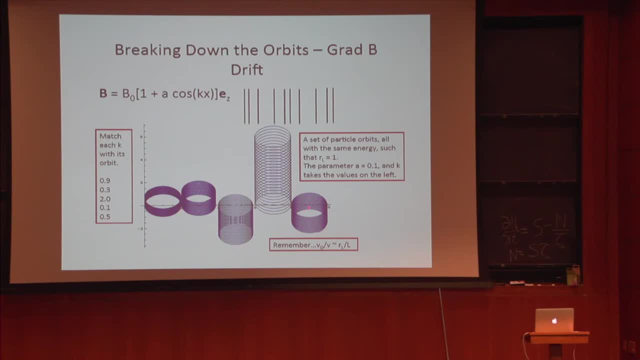 Okay, So the relative, so these all kind of look like springs, like slinkies And what. they're all integrated for the same amount of time, And so the drift is: this particle has the fastest drift and this particle has the slowest. 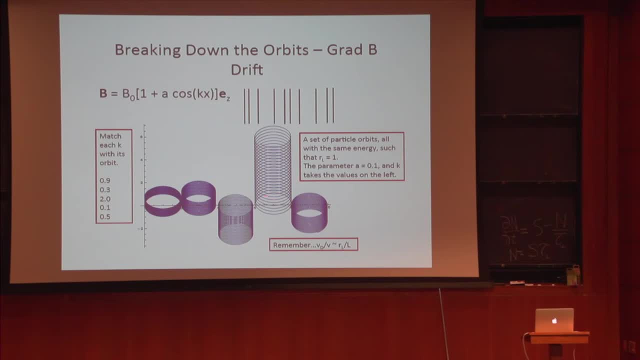 drift, And I want you to tell me which drift goes with which value of k. So which value of k, Which value of k do you think corresponds to the biggest drift? So the amplitude here is: they're all the same, They're all 0.1.. 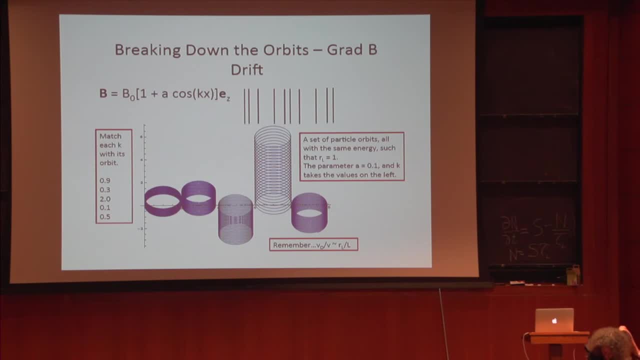 But what about the? what about the k's? How about the smallest drift? The smallest drift should be at pi over, Where the gradient is highest, Where the gradient is highest. Okay, So is it always pi over 2?? So you're right. 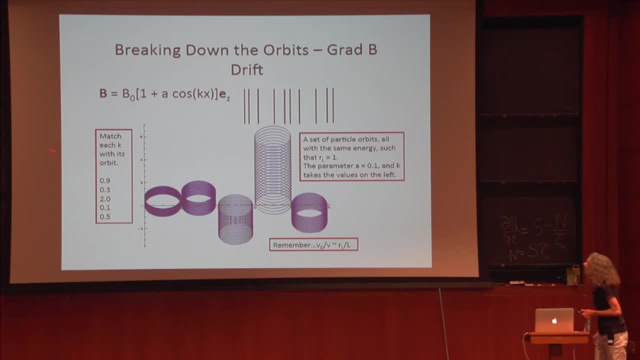 The gradient. so the gradient being high. So let's see, I guess the closest we get to pi over 2 would be 0.9.. Okay, So the larva radius here is 1, and when k is 0.9, that accounts for the largest. 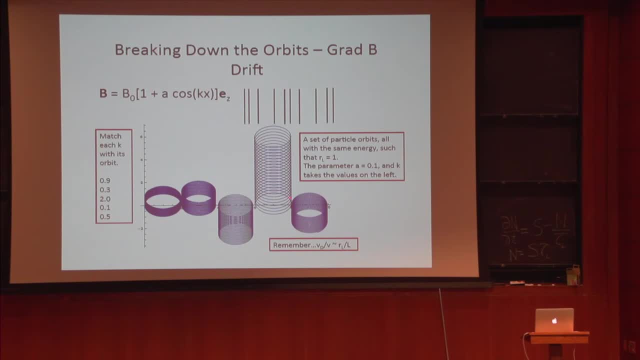 change over this particle's orbit, Where k is 0.1, that represents the smallest change. So for k equals 0.1, the field is practically uniform over the particle orbit and we get very little drift. So okay, so here's 0.1, and then here's 0.3, so we get a little more. 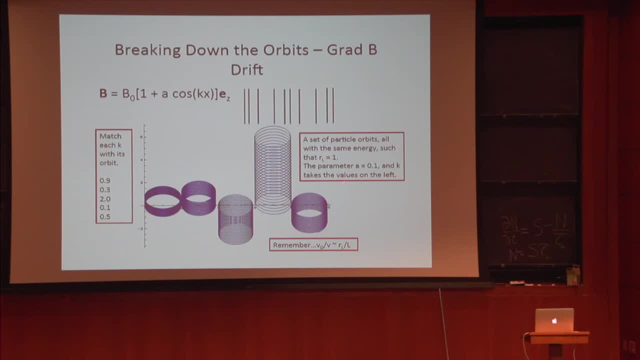 drift. And then here, all these particles have the same larmor orbit size, And then here's 0.5, and then here's 0.9.. And so you might say, okay, great, I'm going to make k really big. So here's what happens if we make k 2, and it gets small again. Why does? 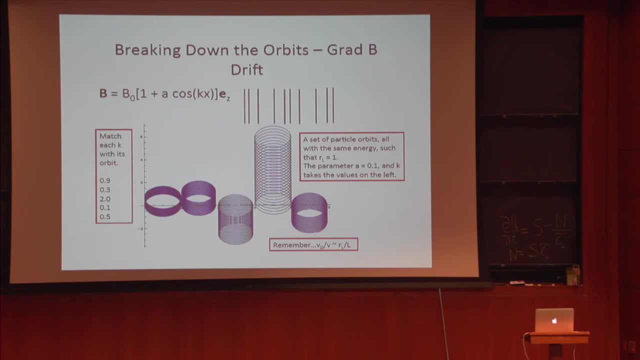 it get small Because if it gets small again, it gets small because the variation in the field actually averages out over the particle orbit. So if we kept making k bigger and bigger, we'd eventually get no drift at all. So the lesson here is that particles interact the most strongly. 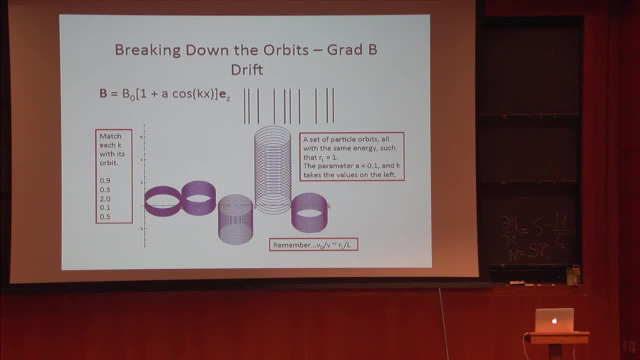 with variations that are kind of on scales comparable to their own gyro orbits: Small-scale variations they don't see. Larger variations they don't see Larger-scale variations they're insensitive to. And a good sort of takeaway message which you can get from doing any kind of drift theory is that the ratio of the drift speed to the 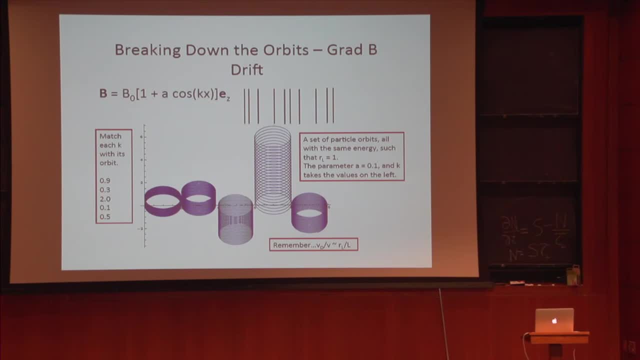 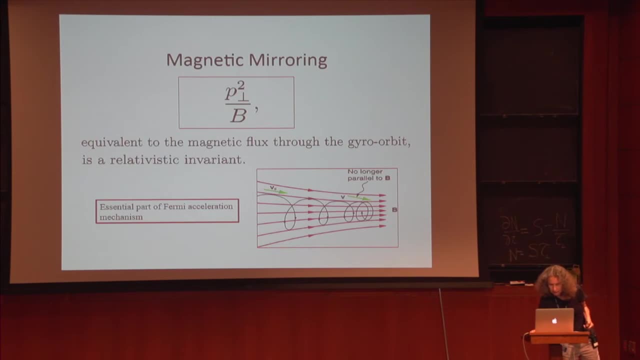 total speed, gyro speed is of order. the larmor radius divided by the scale. Does this all make sense? Okay, Okay, so magnetic mirroring. So the relativistic version of the magnetic moment, adiabatic invariant, is the perpendicular. 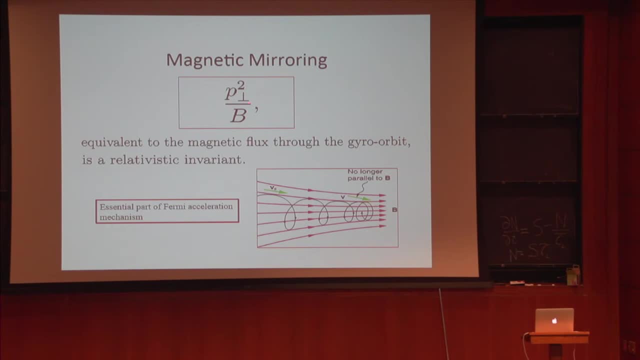 so perpendicular means perpendicular to the field, p, perp squared over b, and that's basically the magnetic flux through the gyro orbit. And so here, if we have these converging magnetic field lines, a particle will spiral around, but the spirals are getting tighter and tighter. 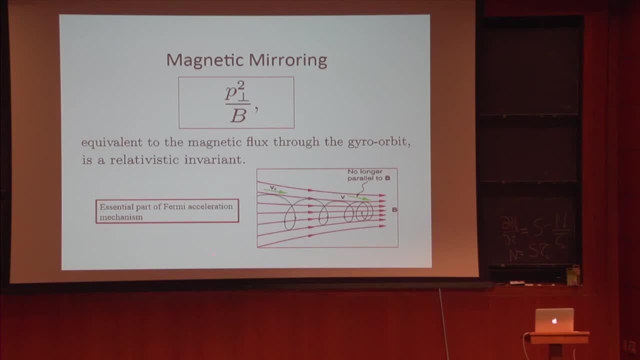 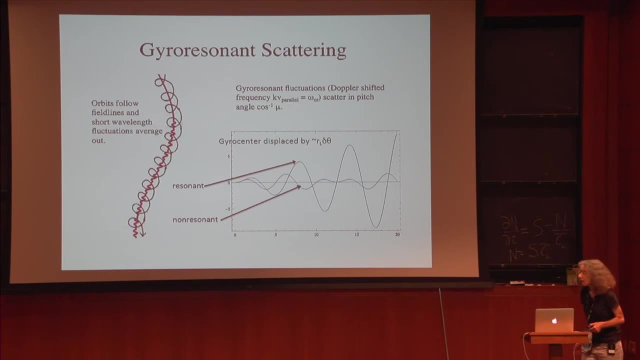 and it will eventually start coming back. And it's good to understand that there's a difference between the two, because it's an essential part of the Fermi acceleration mechanism. Okay, Gyro, resonance scattering, So here is a sketch of a magnetic field line. 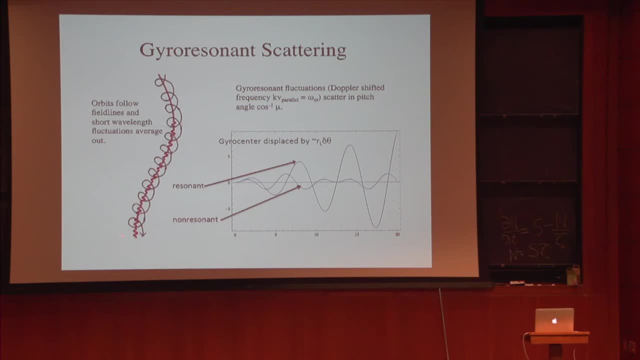 that has that varies on two scales. It's it's got a very kind of long wavelength scale and it's got a very short wavelength scale of variation. And this black line represents the orbit of a particle. So, as you can see, the orbit is following the field line, the 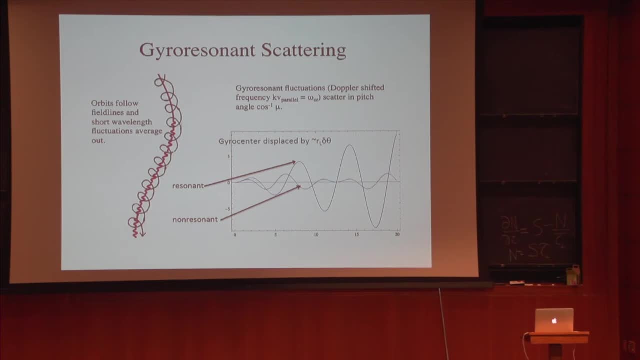 large scale field line very well. So it's kind of like riding your bike up and down the hill And the tiny scale variation it it really barely sees. So that's like riding your bike over kind of washboard. It's makes your hands vibrate a little bit, but you can. 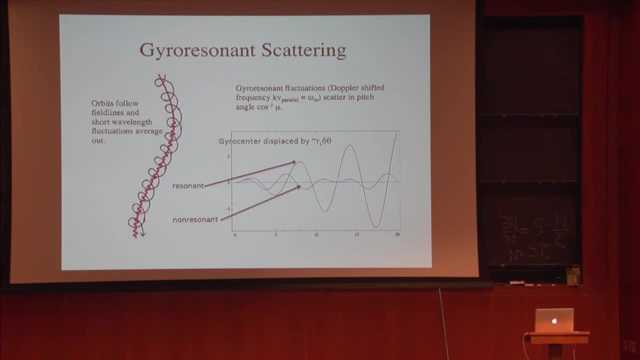 stay on. However, if you encounter a fluctuation that's approximately the length of separation of your bicycle wheels, you will interact very strongly with that fluctuation And I didn't try to draw that, but this is just an orbit integration for a resonant particle and a non-resonant particle And the mathematical 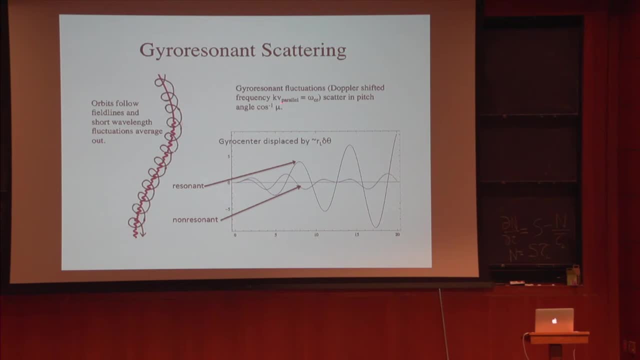 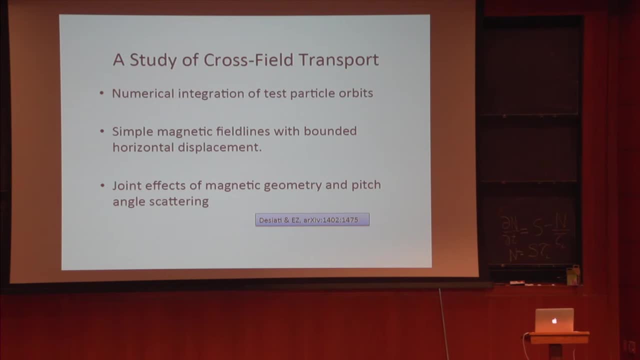 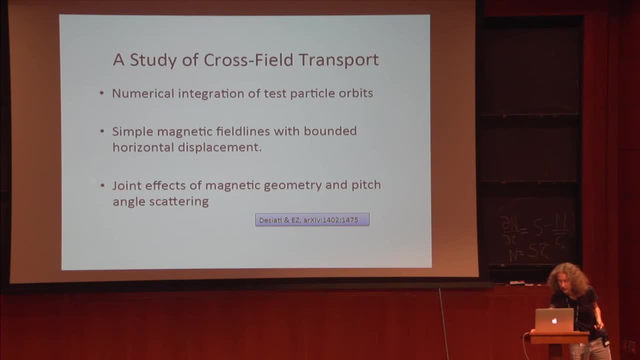 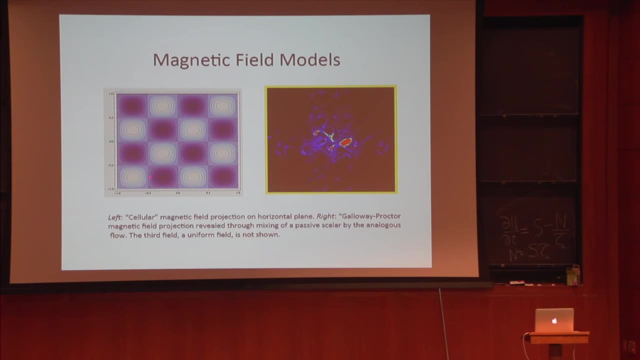 and pitch angle scattering. Okay, so what happens? So the magnetic field models that we chose were ludicrously simple. We've since made them more complicated. I'll say a little bit about that. So there's a dominant component of magnetic field that propagates. sorry, 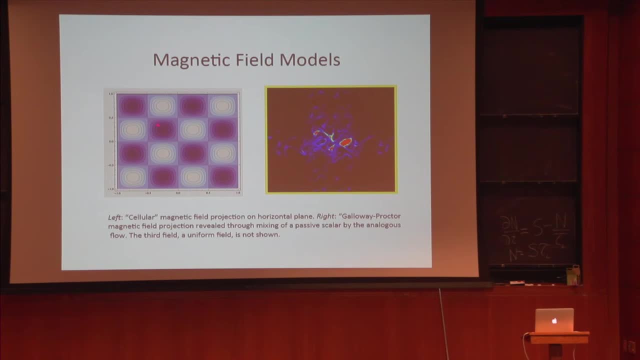 that's oriented perpendicular to the screen, And then if we project the field down on the plane, we have this sort of cellular structure, So the field lines are very weakly wound- helices, kind of like that. And then this is a time-dependent magnetic field model. 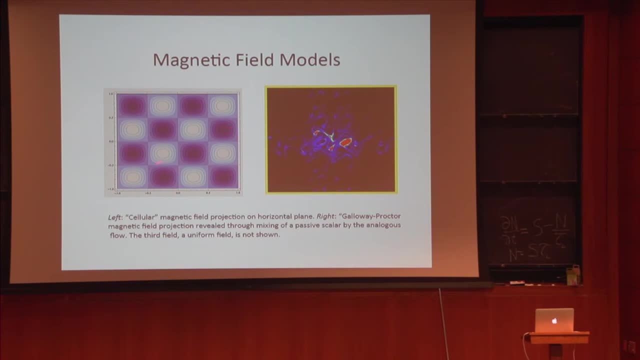 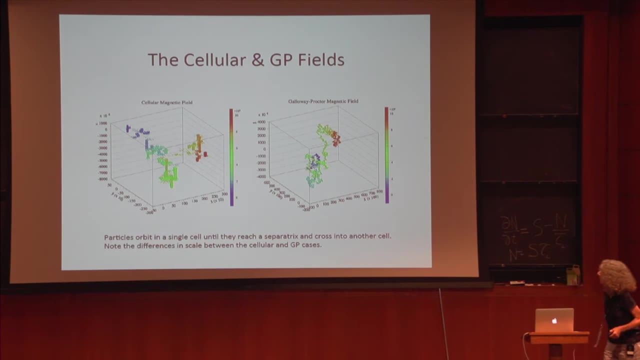 It has a single spatial scale, but these cells kind of waggle back and forth, and that actually leads to chaos, okay, So what do particle orbits in this magnetic field look like? So we implemented pitch angle scattering in a very simple way, which I'll describe later. 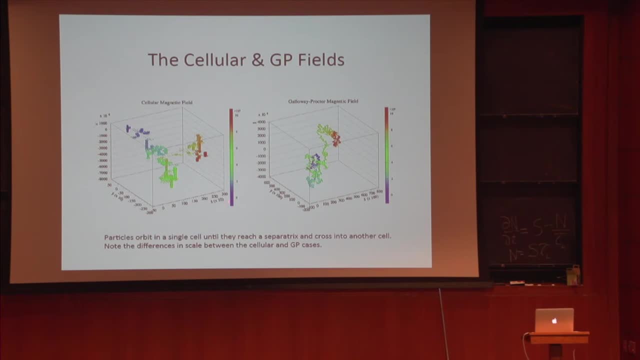 and we let them propagate, and this color coding represents a progression through time, And what happens is magnetic field particles kind of hang out for awhile on a single helix, Okay, but every now and then something happens and they cross over onto another helix. 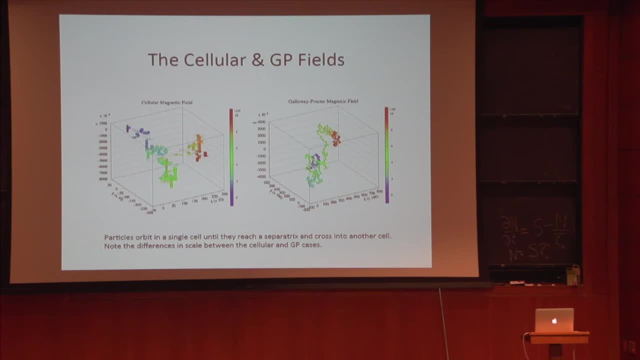 then they hang out on that helix for a while, then they cross over to another helix and so there's a substantial amount of movement from one helix to another. and it's brought about by this pitch, angle scattering and in the time dependent field they really never stay in any helix for very long. the helices 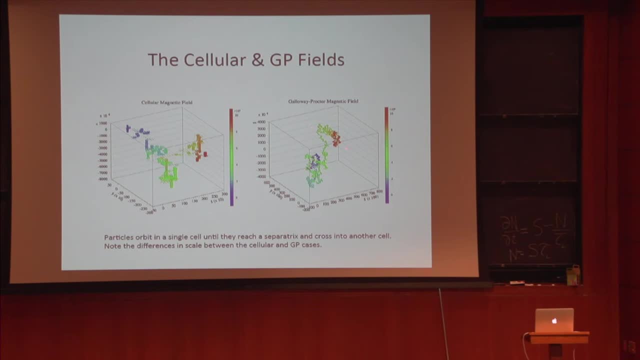 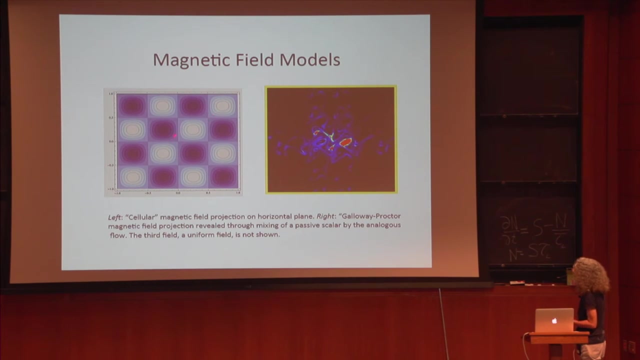 are constantly moving and we get a very chaotic trajectory. yeah, it's a bit like a standing wave. so if we go back to this, this picture, then what would happen is that these, these cells would be kind of wagging back and forth, and so, as you probably know, there's no chaos in two dimensions if you have a steady. 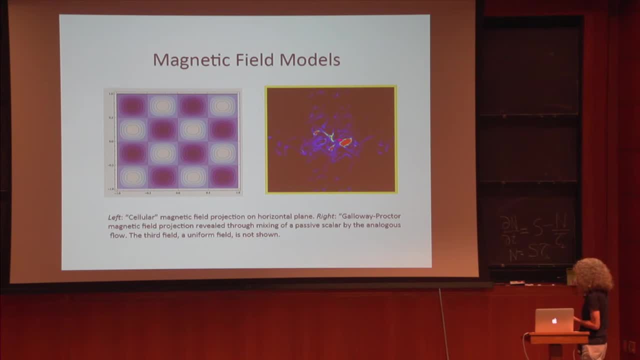 flow, but if you have an unsteady flow, there's there's lots of chaos and what this color represents. so so I don't really have the nerve to try to show movies of this field, but this shows what happens if you lay down a passive scalar on this field, and what happens is that it very, very quickly disperses. so 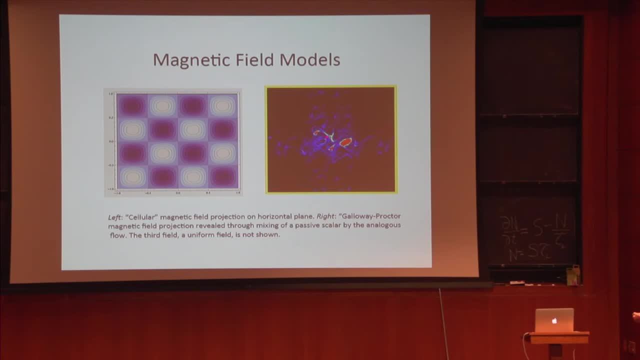 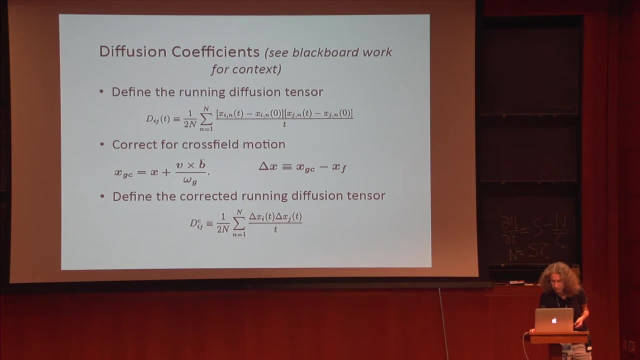 we started with. you know, kind of a white circle here, and everything just gets thrown around very quickly, and the same thing happens to these particles. okay, so can we try to quantify this transport? so in order to do that, we define a so called running diffusion tensor, and it's so, it's a. 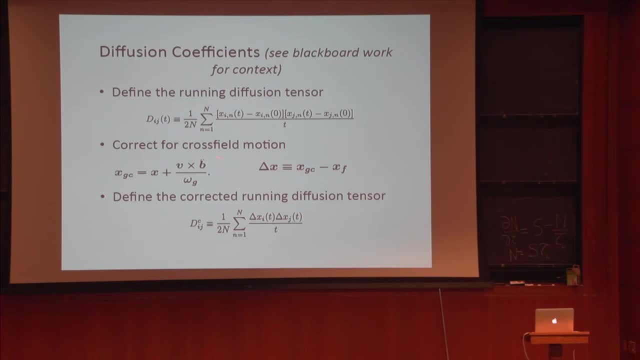 tensor. it has two indices, and the ijth component of the diffusion tensor is 1 over the number of particles. so we typically have 1,000 particles in the ensemble, and so we look at the displacement of the nth particle in time relative to its original position. we do it for the ith component. 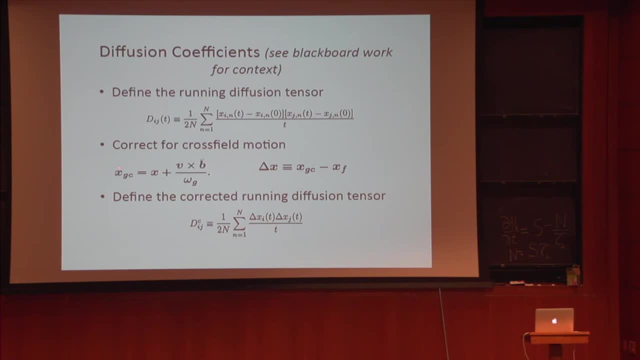 and the jth component and we divide by time, and then we apply a correction that accounts for motion of the gyro center and that turns out not to make a very big difference. but that's what I'll be showing you. Okay, so what does that look like? 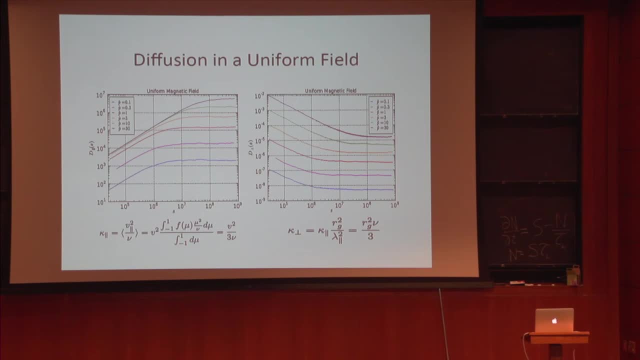 So this is what happens if we have pitch angle scattering in a uniform field. We're going to derive this expression later. I think we'll get to it today. So here is the parallel diffusivity, and here's the perpendicular diffusivity, and let's 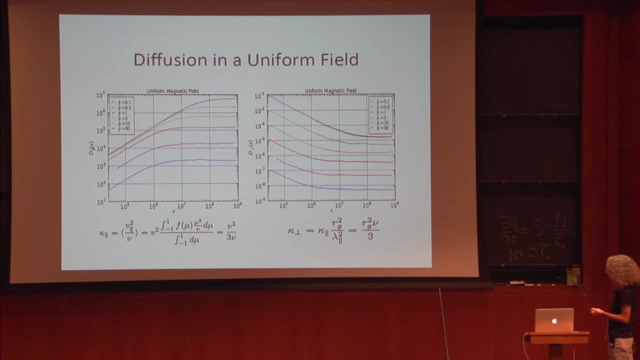 So the perpendicular diffusivity is much, much smaller than the parallel diffusivity. These colors here represent particles with different momenta. So the parallel diffusivity, The parallel diffusivity, increases for a while, and then it levels off at some value. 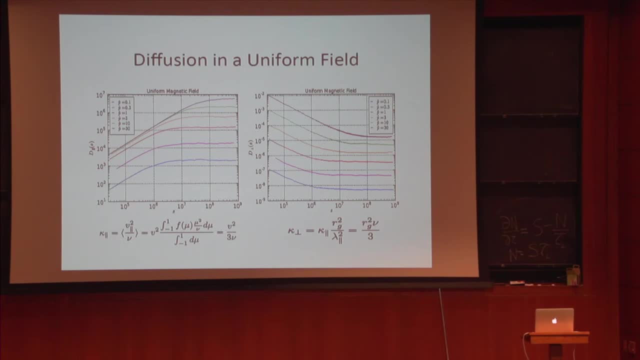 And what does that mean? So if we think of that running diffusion as basically delta x squared over t, if delta x squared increases as t, like it does for sort of a standard random walk, then it should be a constant. If delta x squared. 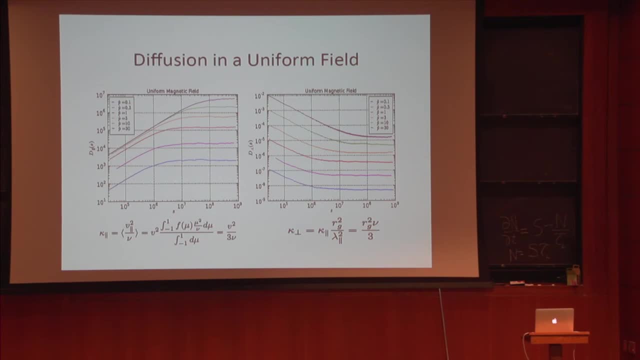 If delta x, squared, grows more slowly than t, then it will decrease, and if it grows more quickly than t, it will increase. So really all possibilities are covered, And what we see for parallel diffusion is that it increases for a while and that just. 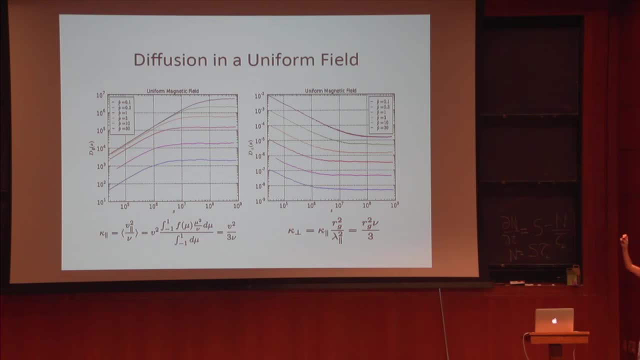 represents particle motion along the magnetic field until it scatters. But eventually the scattering brings it back and it has a random walk-like behavior. So this actually works Okay. And then the perpendicular diffusion is the opposite, So the particles are just sort of gyrating for a long time. 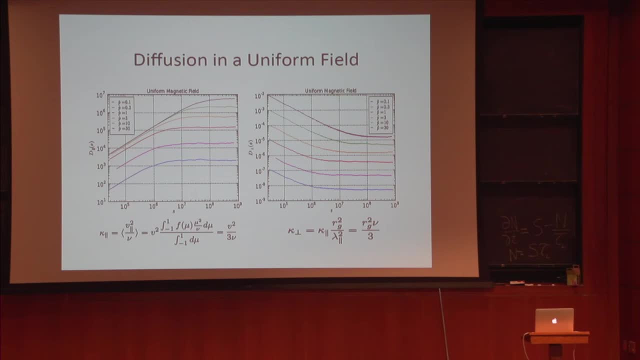 They're not going very far. but time is increasing and that brings the diffusion coefficient down. But again it levels off at some value And here's an analytical derivation of those two values. So we're going to derive this. We're not going to derive this. 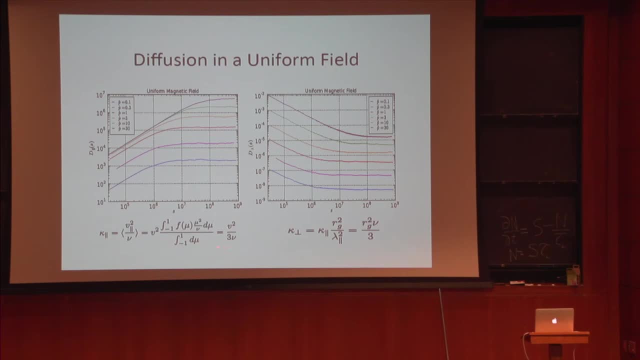 So the parallel diffusivity is v squared over 3, nu, and the perpendicular diffusivity is down from the parallel diffusivity by a factor of order: the gyro radius divided by the mean free path squared, which is typically a very small number. 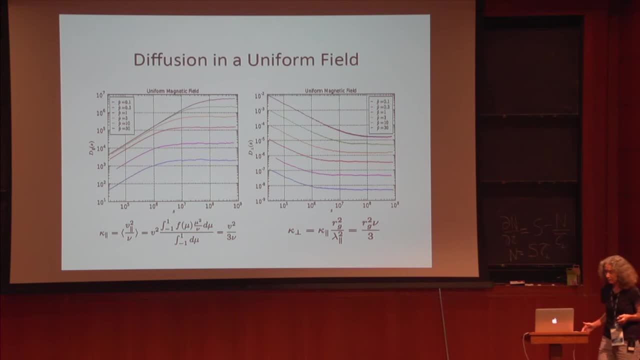 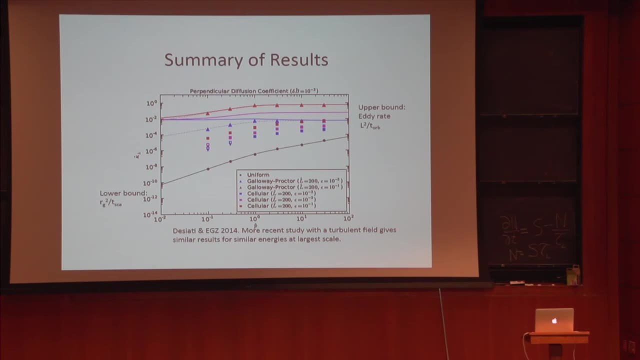 So these particles are really well stuck to their magnetic field lines. But when we combine Pitch angle scattering with this magnetic geometry we get a pretty big enhancement of diffusion. And we What we argued in our paper is that the diffusion is bracketed by two extremes. 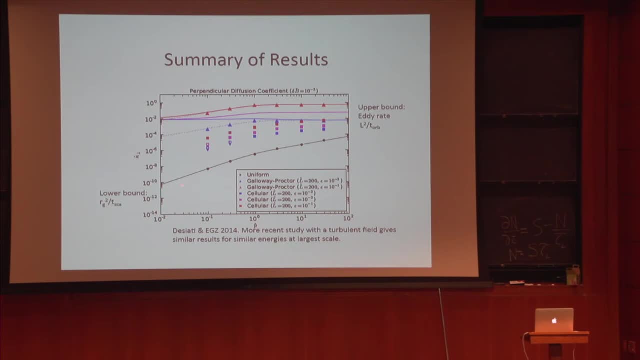 So this is the lower bound on the diffusion. This is the formula that you saw. This is as a function of momentum And basically it increases with momentum, because the gyro radius increases with momentum And the upper bound is kind of an eddy diffusion. 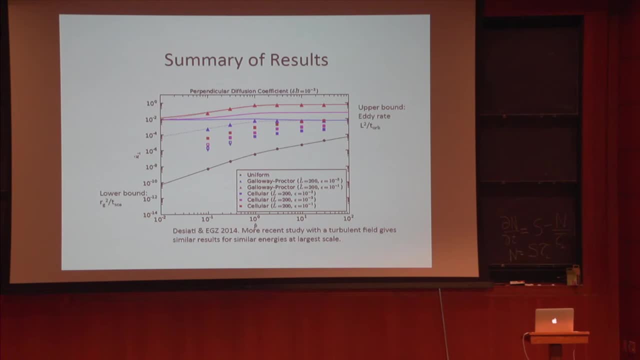 It's what would happen if a particle- Every time a particle- circulated once around a helix, it crossed over to another helix, So it's sort of the maximum rate at which it could migrate as it goes around these helices, And that upper bound is very close to being achieved for this time-dependent field. 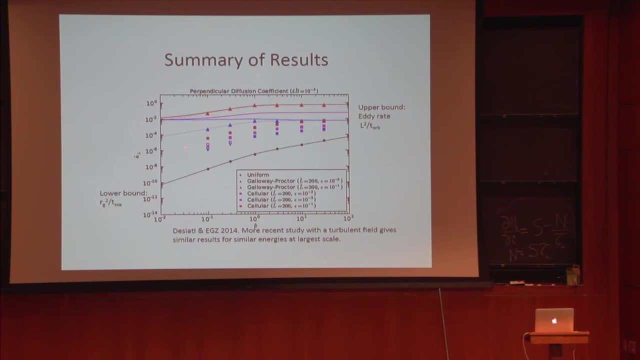 But for this time-dependent field it's very close to being achieved. for this time-dependent field, But for this cellular field that's sort of stuck in between. So the fields that we chose were so simple that we weren't sure this result had a lot. 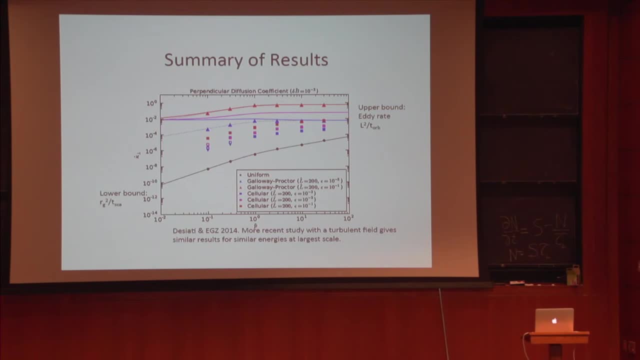 of universality. So more recently we've been working with a turbulent field. So instead of nice regular cells we have sort of protozoa-like eddies, But the same basic structure is maintained And that's what we're trying to do. 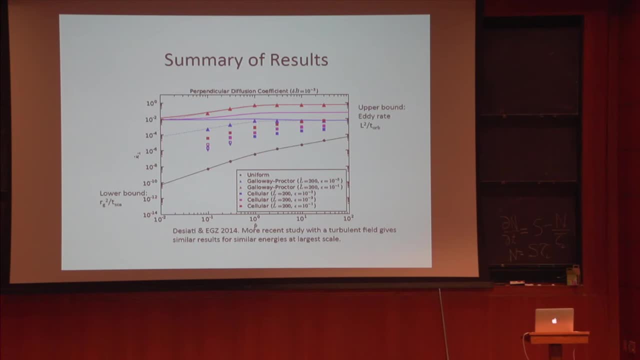 And that's what we're trying to do, In the sense that particles tend to. Space is sort of divided into cells, even though they're cells with funny shapes. A cell is defined by magnetic field lines winding around a single axis, And then there are these separatrices that divide the cells. 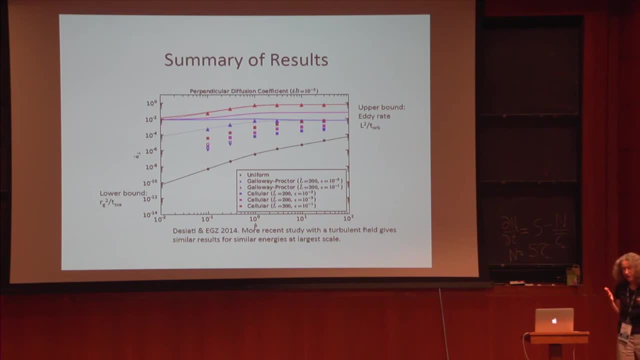 And what we found is that if the energy in the largest cell is about the same as the energy in the single cell and they're the same size- then the diffusion rate is going to be about the same. And if the energy in the smaller cell has the same amount of energy, or if it's about 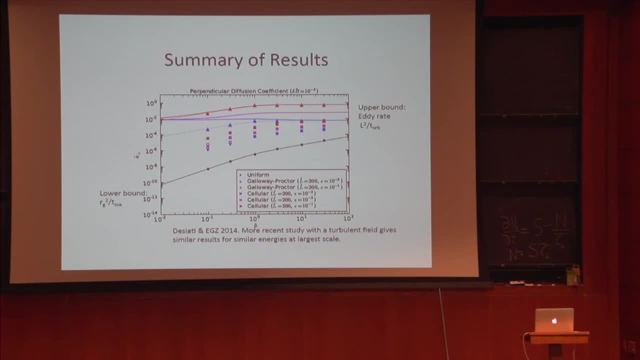 the same amount of energy. that means that the diffusion rate is going to be more than the amount of energy, And so we decided: well, we're going to go ahead and drive the superior line up a little bit. I want to drive the superior line up. 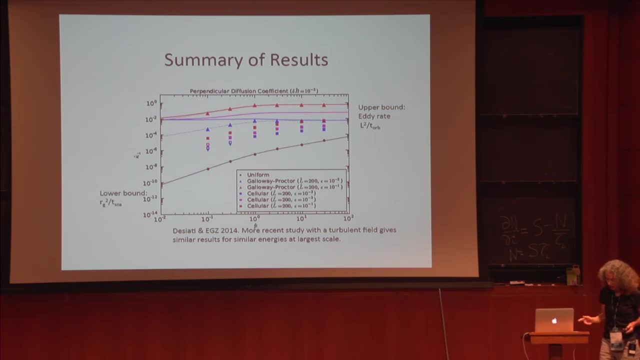 And we wanted the lower line up to allow for that. So we took the upper line up and then we took the lower line up, And then we took the lower line up and we rolled in between the two of them And then we pulled the upper line up a little bit. 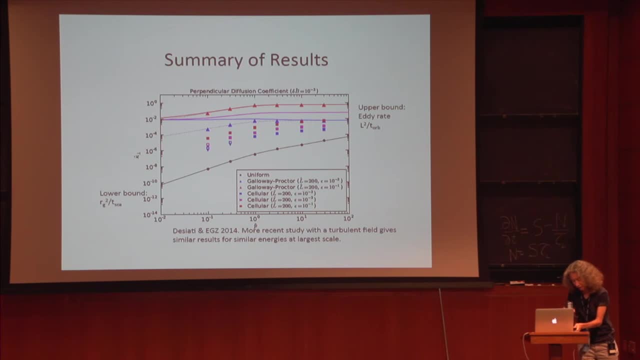 And in the end we ended up providing the lower line, And I think that's all there is to this. So this is also something we called the superposition analysis of the molecular recommendation. So every so we integrated the particle orbits, and then at certain times, we we chose a random. 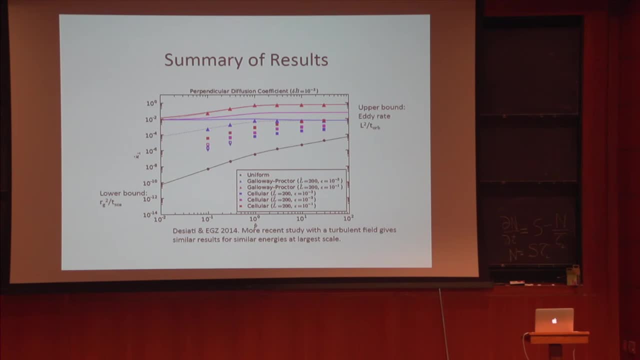 pitch angle: small, very small, pitch angle change of a certain, of a certain amount. Now, now, why would, why would you do something like that? The reason we did it is because of this multi-scale problem, So the fluctuations that are scattering the GEV cosmic rays- we envision this as gyro. 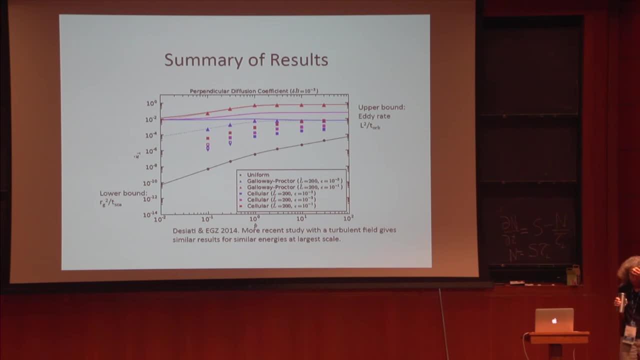 resonance scattering those fluctuations are. you know? they're at maybe a tenth of an AU in size 10 to the 12 centimeters. But the whole galactic magnetic field has structure on scales of parsecs, And so we can't simultaneously simulate both. 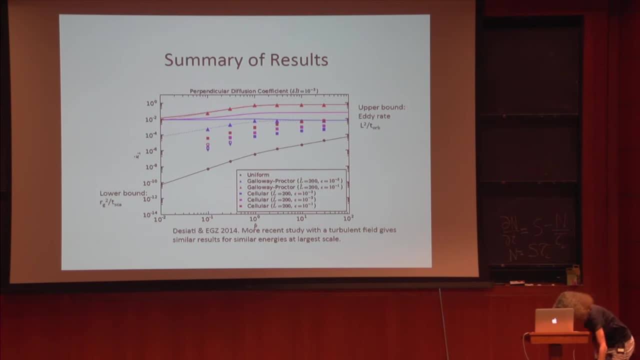 We can't encompass that range of scales. So what we wanted to, what we wanted to be able to show, is that the combination of, or investigate the combination of, magnetic geometry with a little bit of pitch angle scattering facilitates this, this migration across separatrices. 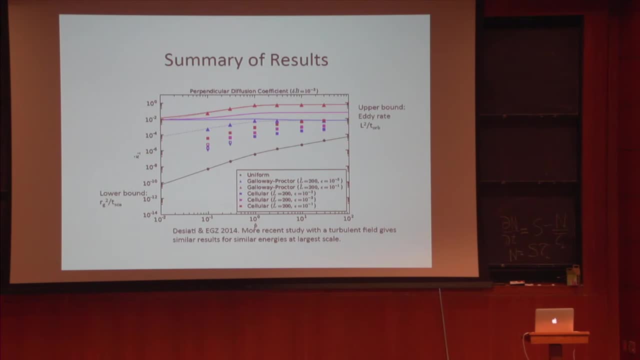 That's really what. that's really what our work shows, and I think it's true, It's intuitively plausible. That's basically. that's basically the idea, But But also so the so the pitch angle scattering is a is a bit of a saving grace as far as 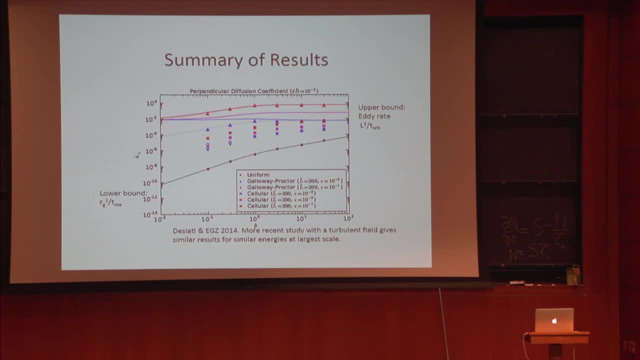 the numerical accuracy is concerned. So you know, we tracked energy, we tracked canonical momentum. They're well conserved, but by kind of resetting the clock with this pitch angle scattering, you don't demand as great accuracy as you would, you know, if you were doing it for 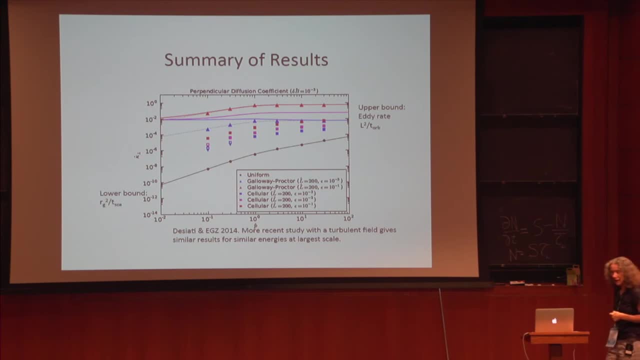 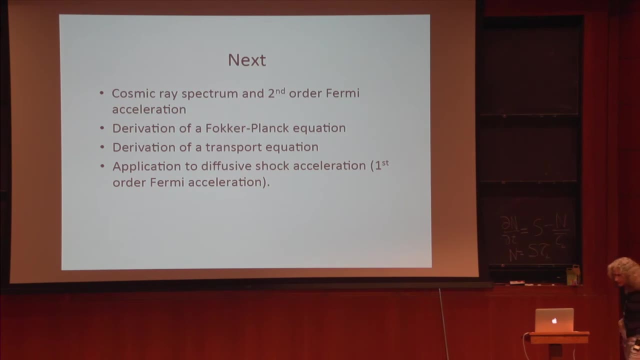 the full 10 million years, Okay, So. so this is. we're now coming to the end of the slides part of this presentation. I'd also like to say I know that there was a talk last week about how you can effectively convey information on slides and as I was, you know, sort of designing my slides, I kept 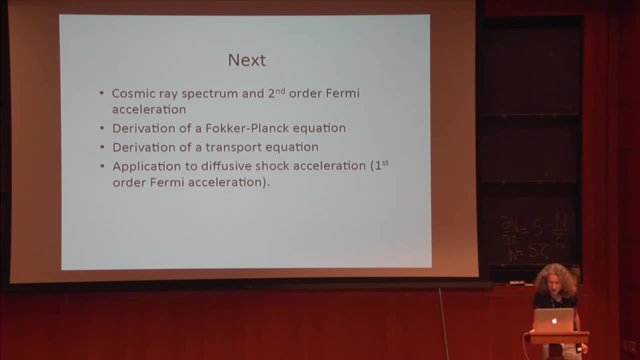 thinking I was violating all the rules, and you all know the rules and I don't know them. But anyway, that's it So. so that's it for the slides. So if you have any questions about the slides, let's talk about them now. 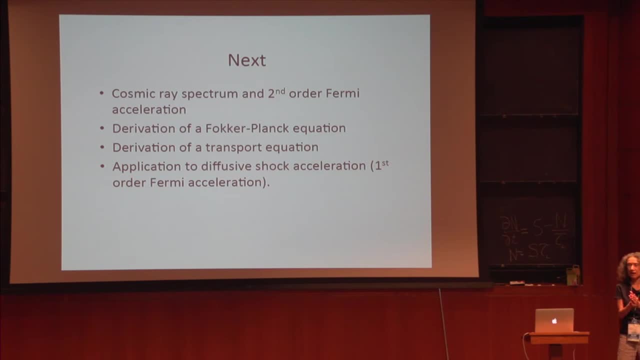 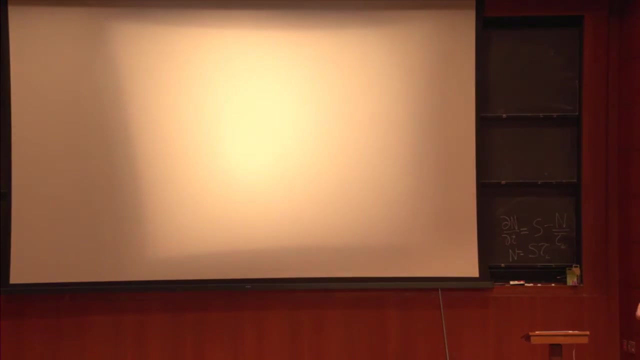 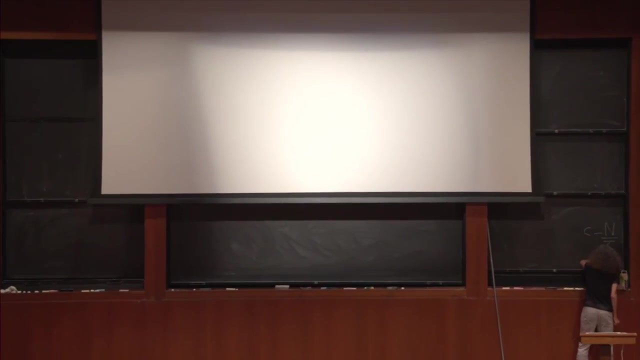 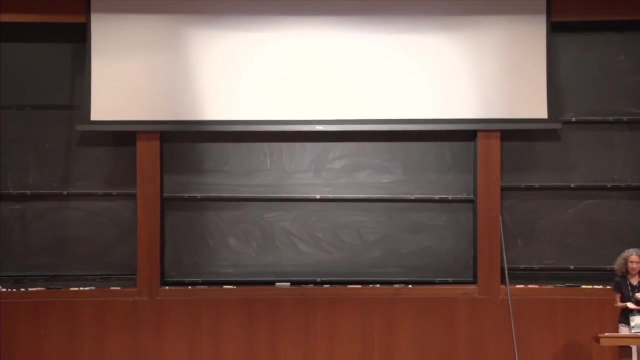 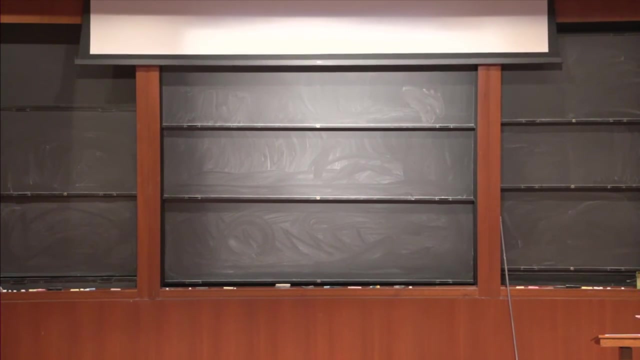 Otherwise we'll retract the blackboard and do some writing. Any questions on this part? Okay, Then. then let's say goodbye to this. Okay, So, let's go back to the slides. Okay, So, so we have some notes. They've been scanned. 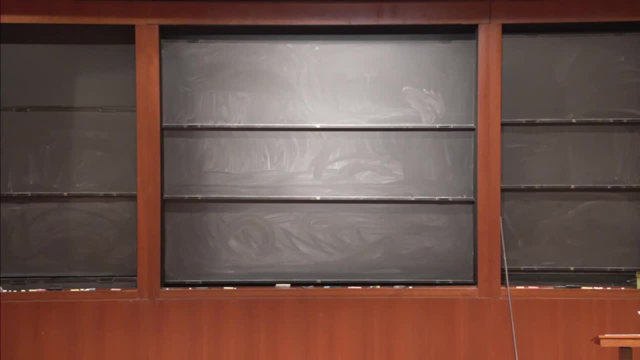 They may be corrected. I decided not to give them to you right away because because my decades of experience in the classroom have taught me that you're more likely to pay attention if you don't have the notes in front of you. So Okay, 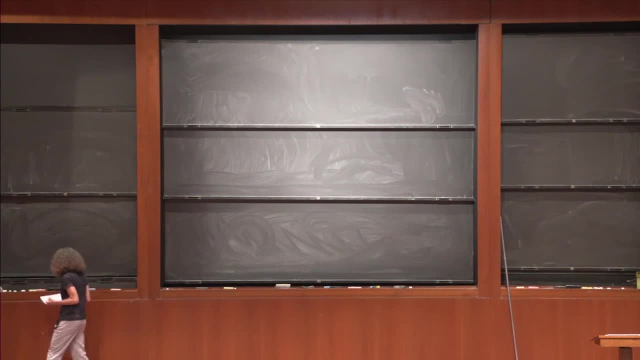 So the the first thing that I'd like to take you through- and you know, all the stuff that I'm going to be talking about for the rest of today- is in the literature It's. most of it is actually in in Kulsrud's book. 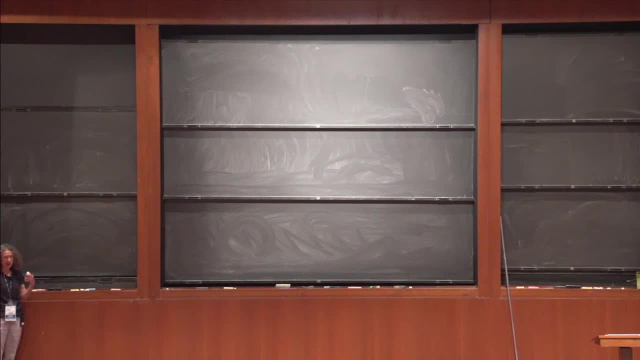 There actually is Kulsrud, Not to put him on the spot, but if you have any questions he can answer them too. But I think it's it's good to just kind of see. Okay, I think it's good to see on the blackboard how this stuff evolves. 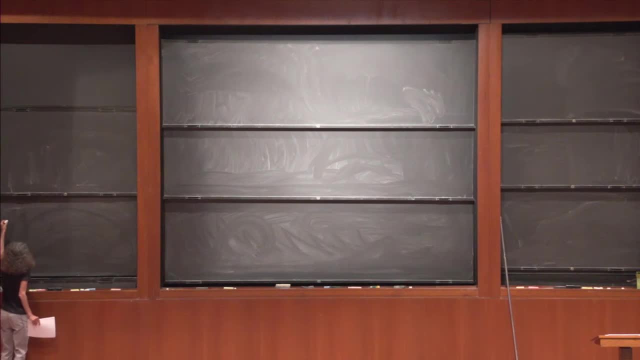 So what we're going to talk about first is is what Fermi did in 1949. So the argument really has has two parts. We're going to talk about a very general way to derive an energy spectrum and then a specific model that gives Fermi's spectrum. 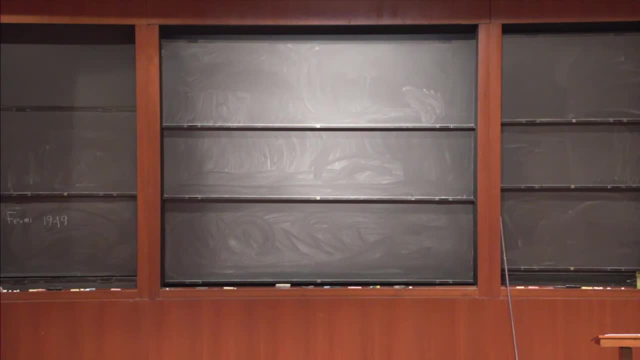 And then we'll talk about whether it's a plausible theory for cosmic ray origin. So let's suppose that particles are injected into our system at some constant rate and they have a constant probability of being lost, And they can. they can be lost by any mechanism that you like. 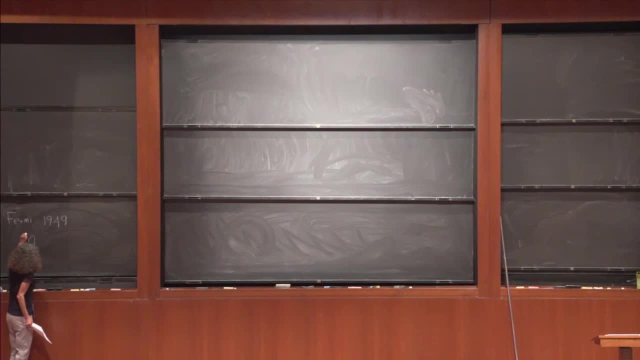 So I'm going to call their distribution n? twiddle Of t, And so n? twiddle of t. dt is the number, density of cosmic rays, particles that have been in the system for a time between t and t, plus delta, t or dt. 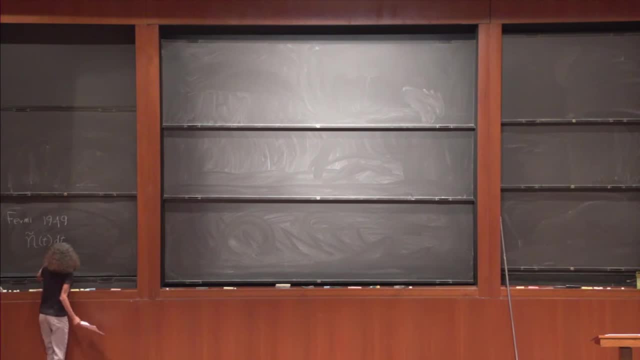 So this is a standard distribution function And it'll be some normalized injection rate times. what Times e to the minus t Over the lost time? Okay, dt, Okay, Can. can you all see this? Am I writing the right size? 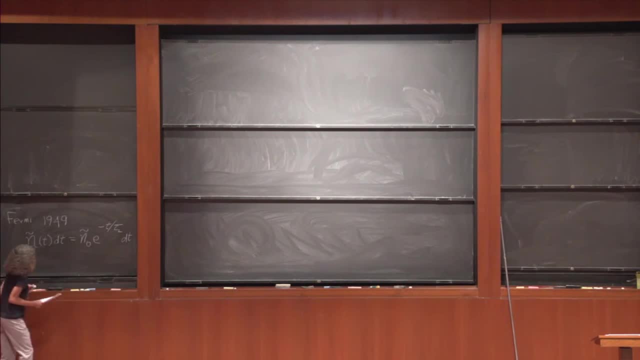 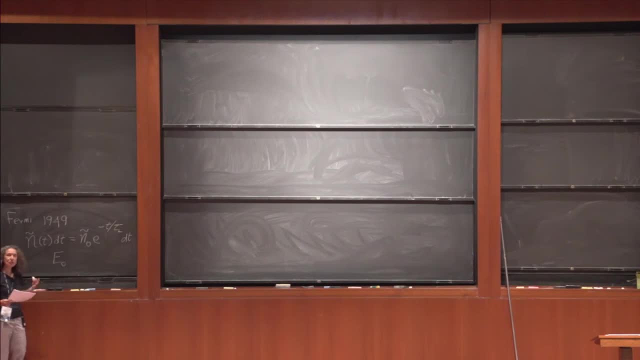 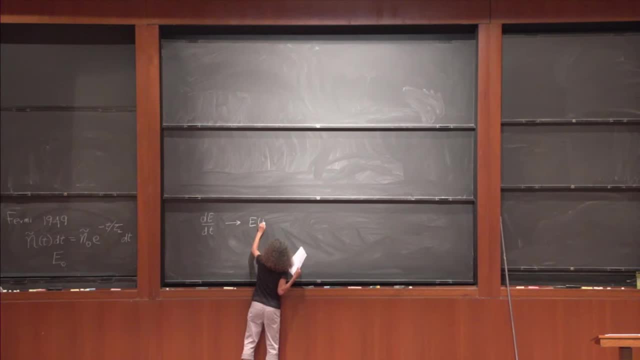 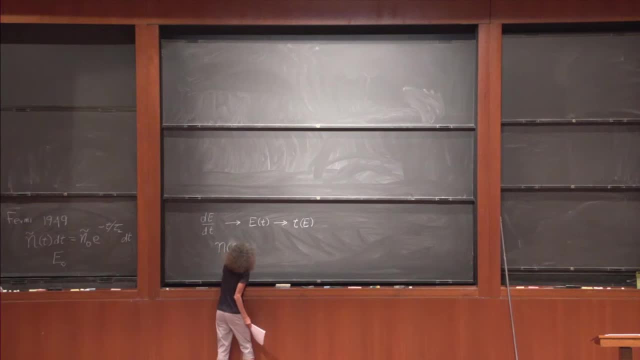 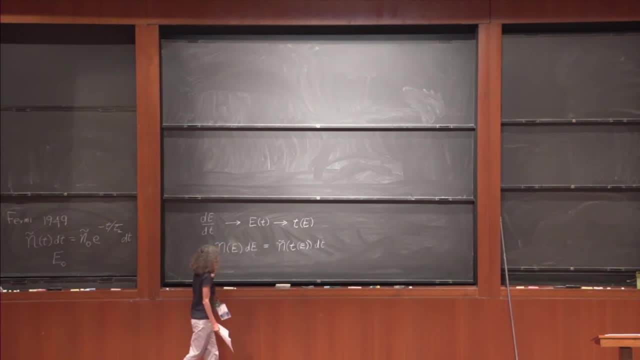 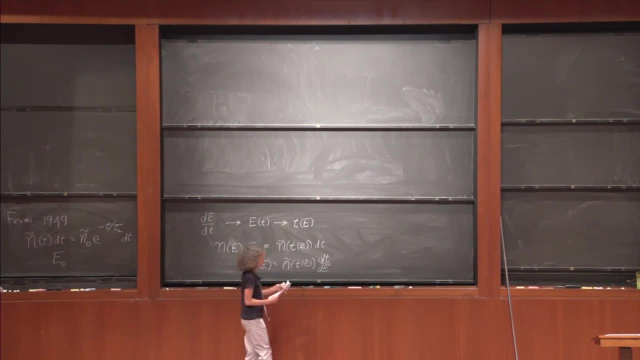 spectrum. OK, So that part is very general. And now let's suppose so Fermi gave this argument and then he made the energy gain law very specific. Let's suppose that d, e by dt, is e divided by some acceleration time. 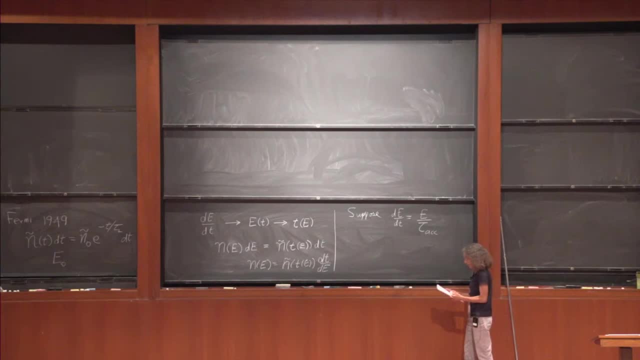 So not every acceleration law will do this, but let's suppose that we have one. So then this equation is very easy to solve. e is just e naught e to the t over tau acceleration, And it's also easy to invert t of e over tau. 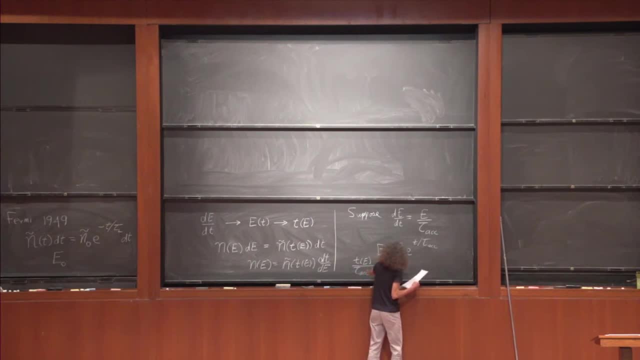 acceleration. So this equation is the log of e over e naught. So if I write down here, can you all see in the back. Good, OK, because I can't go very high. OK, so now let's implement this in this. 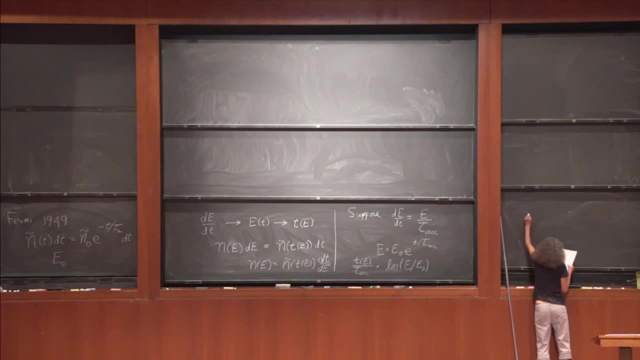 And so what we get is that n of e is n naught. tilde. our injection rate times the acceleration time divided by e naught. So it's dimensionally correct times a power e over e naught. OK. 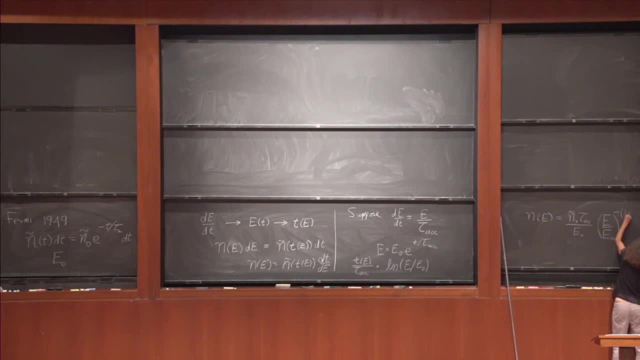 OK, OK, OK, To the minus 1 plus the ratio of the acceleration time to the lost time. OK, so is this reasonable, aside from being dimensionally correct? So what does it say? It says that if the acceleration time is very. 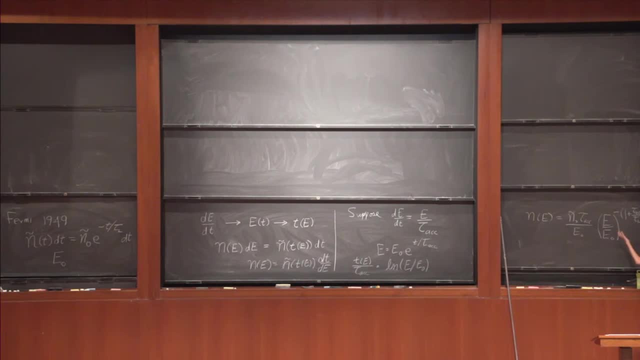 short compared to the lost time, we get a relatively flat spectrum. That makes sense. You have time to get particles up to high energy before they leave the system. But if the lost time is very short compared to the acceleration time, you get a very steep spectrum. 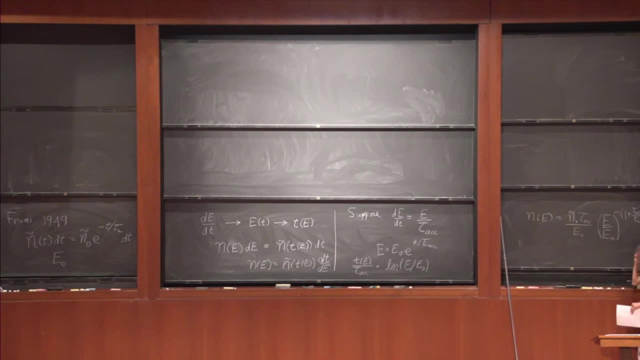 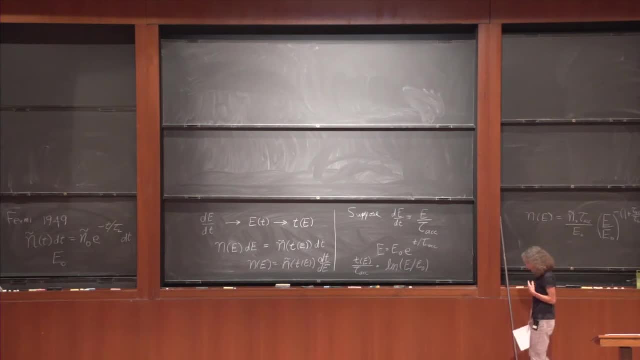 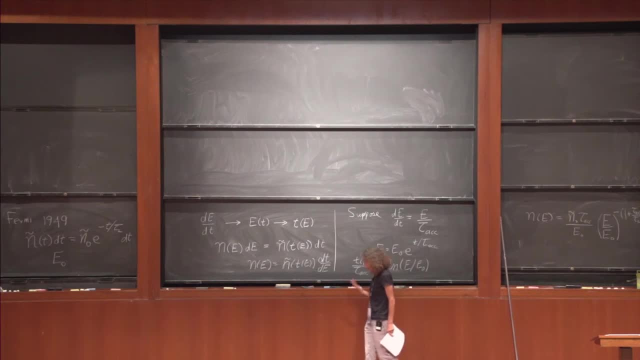 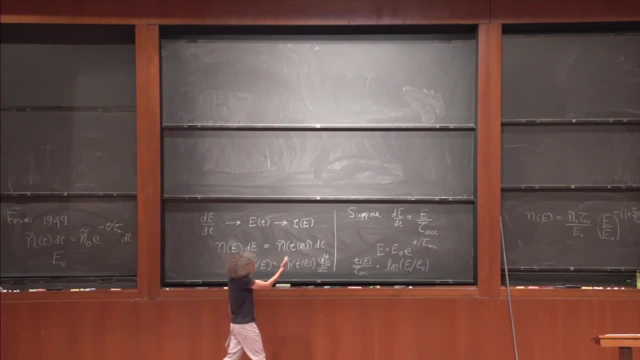 BETWEEN THE DISTRIBUTED SOURCE, SOMETHING LIKE THIS, OR THE DISCRETE SOURCE. Well, there is. so that's a hint. So we showed, by looking at the light element abundances as a function of energy, that the confinement time of high-energy cosmic rays is shorter than the confinement time of low-energy. 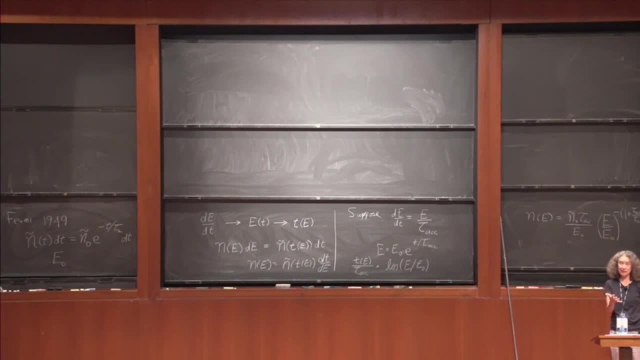 cosmic rays, So the high-energy cosmic rays are younger than the low-energy cosmic rays. On the other hand, in this model the oldest cosmic rays are also the most energetic, And that's the opposite to what we see in the galaxy. In the galaxy, the youngest cosmic rays are the most energetic, and this model predicts: 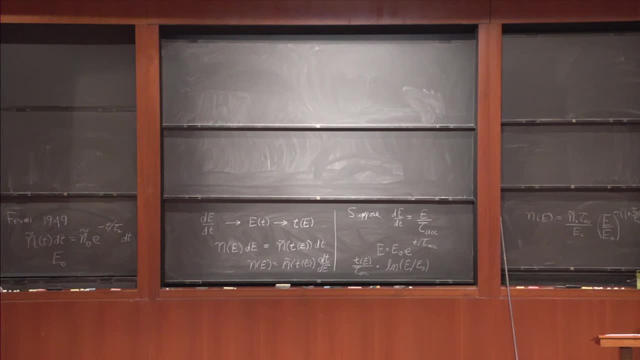 that the oldest cosmic rays are the most energetic. So this is an argument against distributed acceleration in the Milky Way. Okay, So on the other hand, maybe it's what goes on in many other objects And maybe it is, But there's another issue. 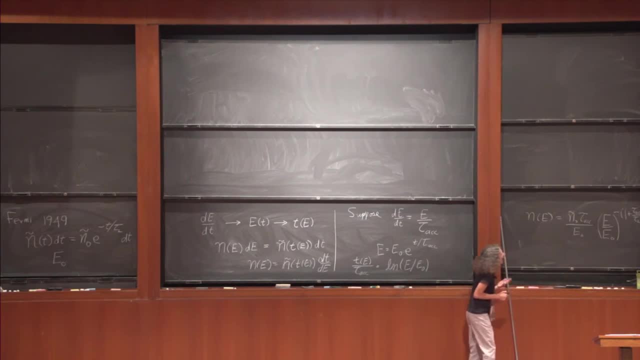 Which is that we know from looking at other galaxies that cosmic ray spectra across the universe seem to be pretty similar. They all seem to be about e to the minus two point something, And that means that this ratio of the acceleration time to the lost time is always about the. 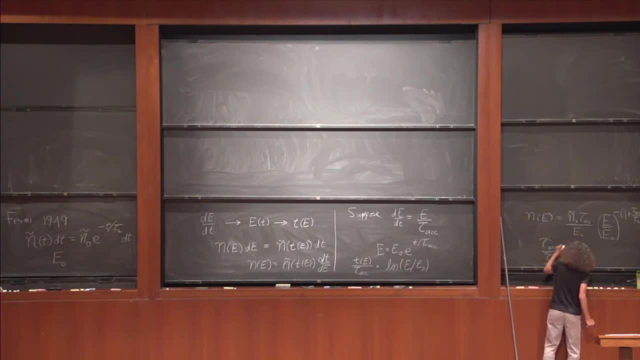 same, And it's always one A little bit bigger than one- Okay, Very close to one. So why should that be? There are so many different things that can cause loss and so many different things that can cause acceleration, So you will sometimes hear that this Fermi mechanism suffers from a fine-tuning problem. 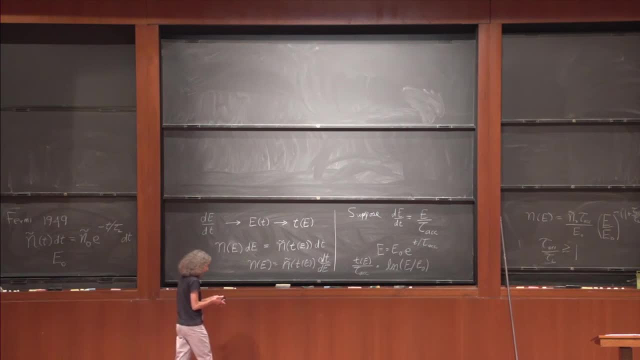 in the sense that you can match the spectrum if you choose the right ratio. But the question is: what should be the basis for choosing that ratio? As we'll see later on, Diffusive shock acceleration, which is not exactly this but close to it, actually predicts. 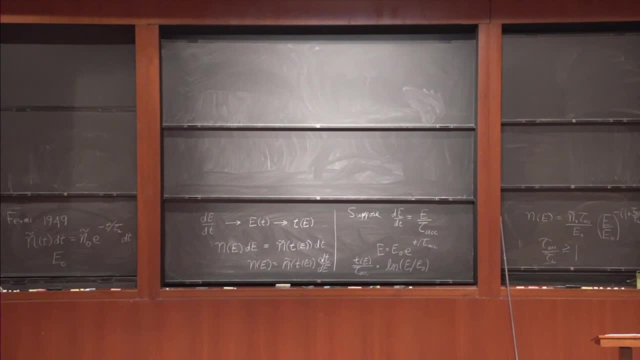 that the acceleration and lost times are about the same. So it's nicely consistent with this model. But now let's go back to Fermi's theory for what the acceleration time actually is. So is it clear, kind of, how this all worked and what the problems are. 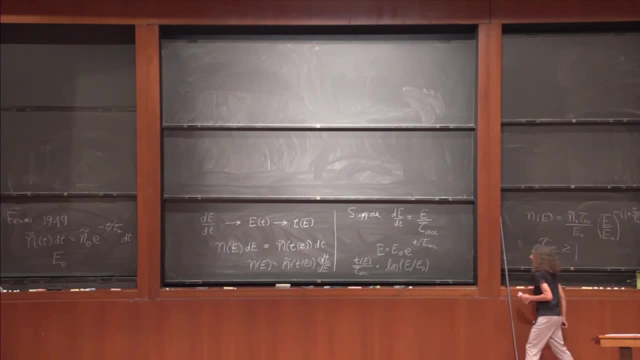 Okay, Okay, Okay, Oh, my God, it's lost forever. Okay, So now we're going to work on the acceleration time. So, Fermi, if you read Fermi's paper, He talks about something called magnetic clouds. picture is that you have the interstellar magnetic field and there are these sort of 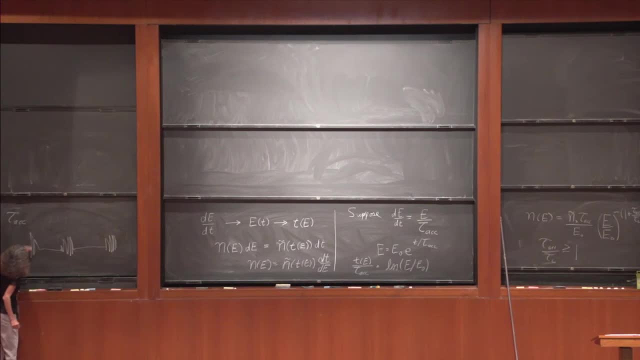 objects on it that are moving around at random and particles. so particles kind of get trapped, They can scatter off one cloud and then maybe they pass through another and they get accelerated somewhere like this and these clouds are moving back and forth kind of at random and 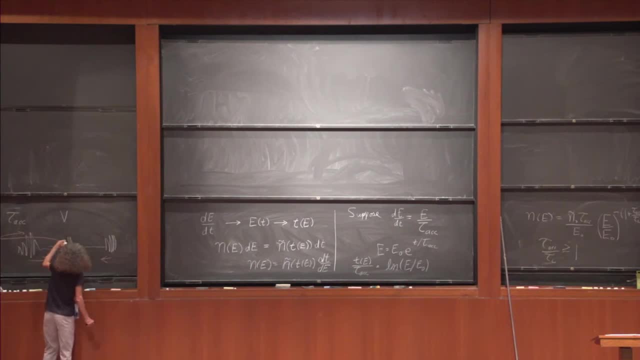 they have some velocity v, some speed v, which can be observed at some characteristic speed for the interstellar medium, probably about 10 kilometers a second. and when a particle reflects off a moving mirror, it either gains or loses energy, Just like hitting a bus. 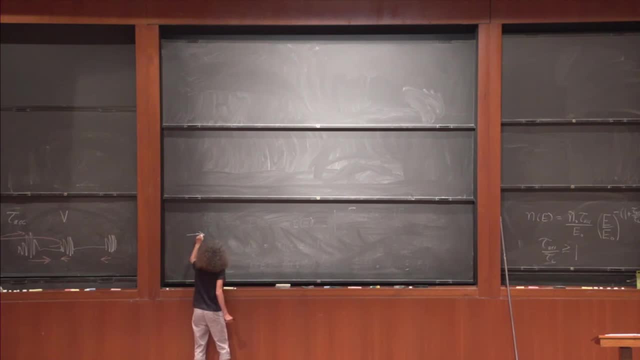 So here's our cosmic ray and here's our moving mirror. and in the case of a head-on collision, so we'll call this the head-on case- If the cosmic ray had momentum p and the mirror, the cloud, had velocity v, then delta. 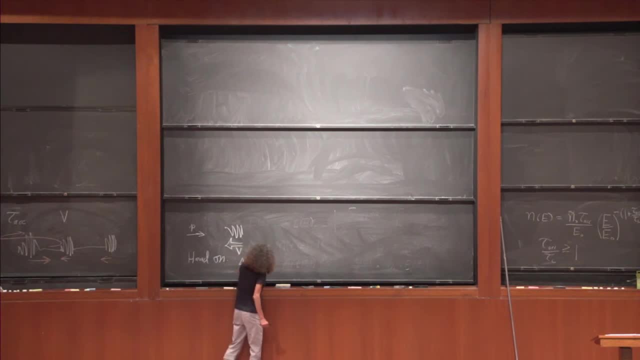 e is positive. It's twice the momentum times the velocity. But if the cosmic ray overtakes a mirror, which is motion p, then delta e is positive. This is what is called the paraccelarity of the mirror. What's the paraccelarity of a mirror? It's the distance. Okay, So we have that. We're going to call that theガql. Anyway, if you're going to calculate delta e, if delta e is positive, it's twice the momentum times the velocity, What's the opposite? 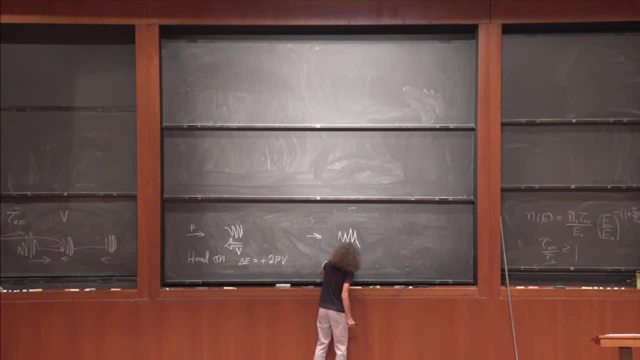 Well, if it's the mirror's momentum, that's why it's positive. If you're going to calculate delta e, then the mirror's momentum is positive, which is moving away. So I'm going to refer persistently to head-on and 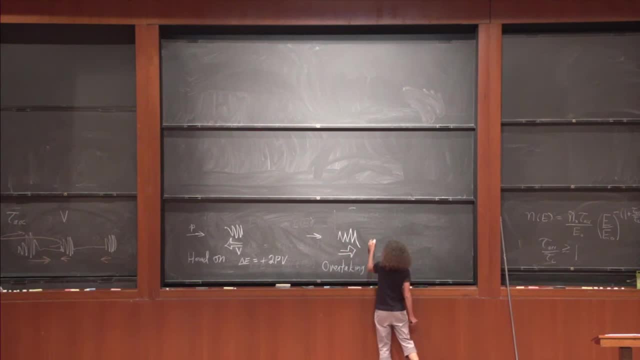 overtaking. That's why I'm writing them down. Then the particle loses energy. delta E is minus 2 PV. OK, so if these clouds are moving around at random, we might think that there can't be any net gain of energy. 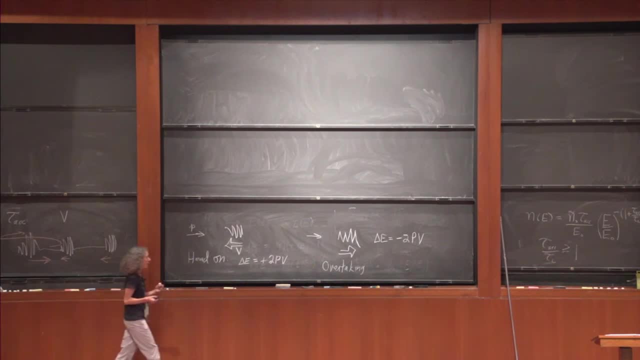 At best there can be some sort of diffusion or random walk in energy space. But that's not quite the case. because if we assume that the mean separation between these guys is L, so the separation between the clouds on average is L, Then the frequency of these collisions will be the speed of 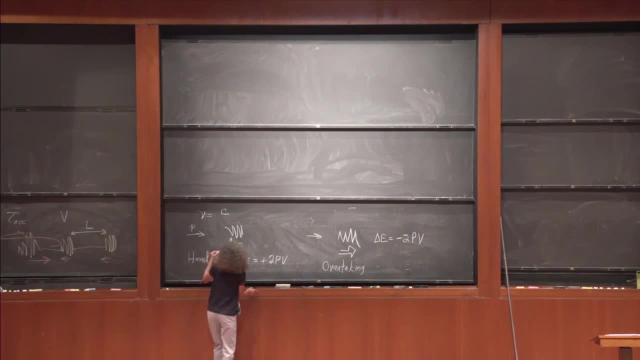 the cosmic ray, which I'm just going to take to be the speed of light plus V divided by L, And the frequency of these I'm just going to take to be the speed of light will be C minus V divided by L. So it takes just a little longer to catch. 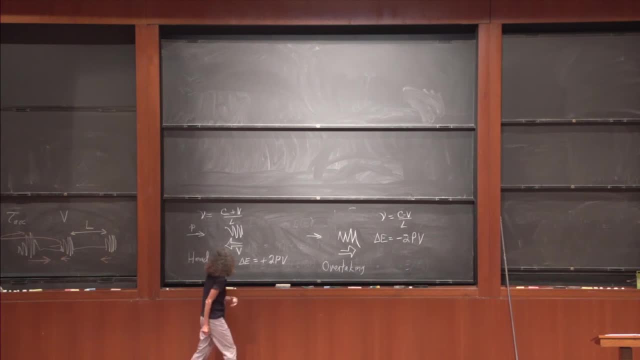 up with the overtaking collisions than for the head-on collisions. OK, so then, if we sum over a lot of collisions, the EDT- I'm going to write it down- It should be something like 2 PV. so that's the energy per. 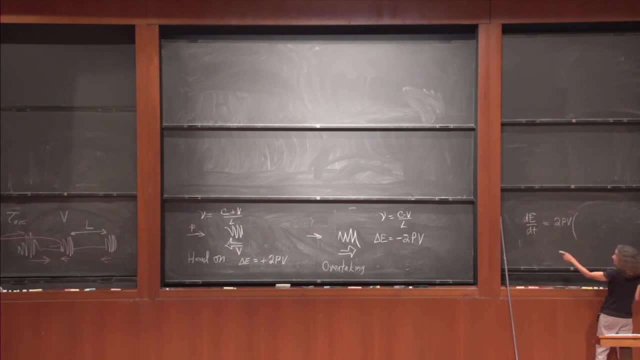 collision times: the frequency of the energy-gaining collisions: C plus V over L, minus the frequency of the overtaking collisions, which is C minus V over L, And the Cs cancel but the Vs don't, and so we get 4 PV squared. 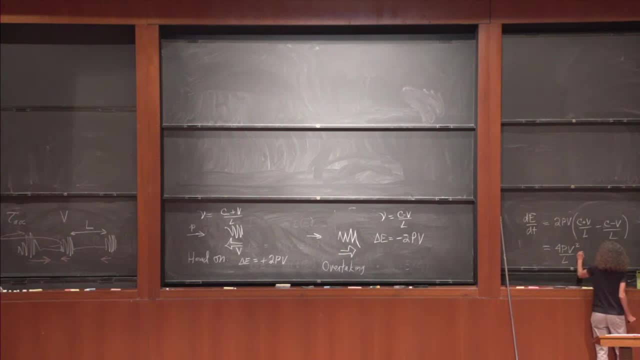 over L, which we can write as 4, so P is E over C, 4 E over C, squared V, squared C over L, We actually do get an energy-gain equation of the form that we needed to derive a power law spectrum. 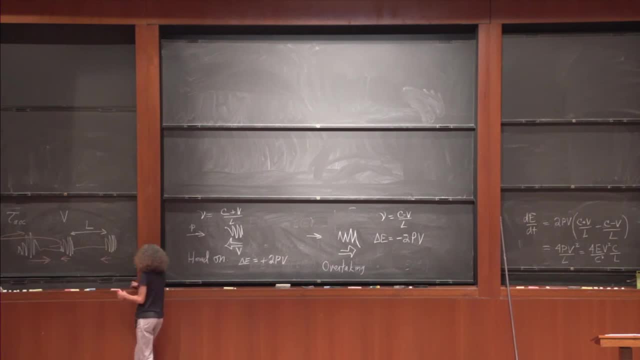 So let's rewrite that And let's also not take this factor of 4 here too seriously, because we should do some sort of Why am I holding this? We should do some sort of average over the relative angles between the cosmic rays and the mirror. so there'll be. 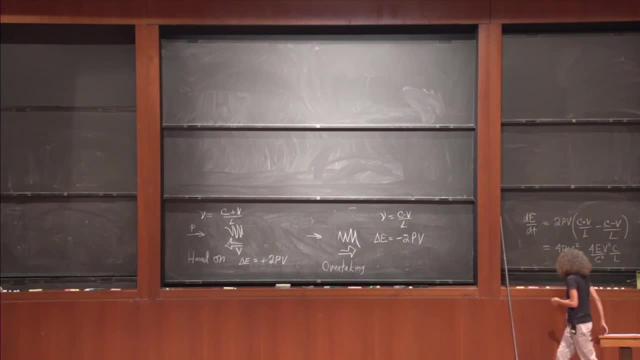 some other number in there of order unity. So we get an equation of the form: dEDT is E over an acceleration time and the acceleration time. So we have our eigenvalue of f and it would be righteousness E over l E2.. 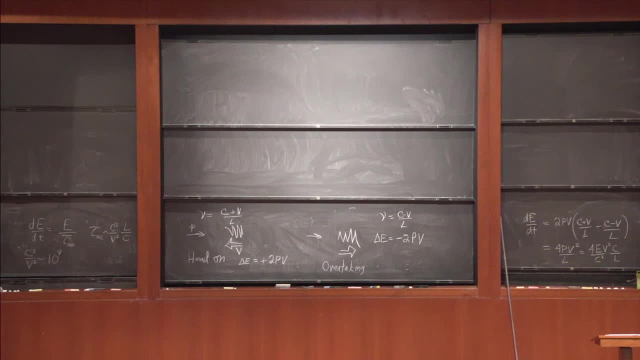 That's the go it. Thank you, Thanks, Good job, Thank you, See you Bye-bye. The duration between clouds is maybe 100 parsecs, So L would be about 3 times 10 to the 20th centimeters. 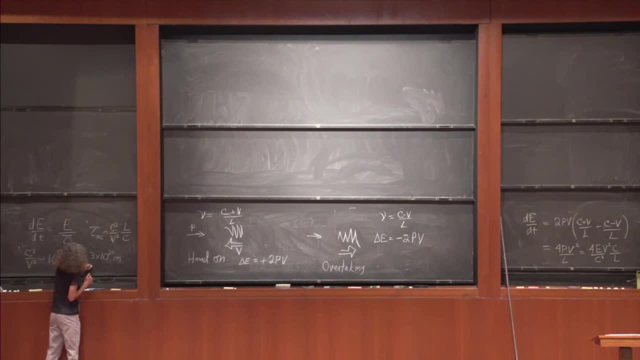 And, of course, C is 3 times 10 to the 10.. So, if we put all this stuff together, the acceleration time is 10 to the 19 seconds, which is 10 to the 19. Isn't it, Yep? which is about 3 times 10 to the 11 years. 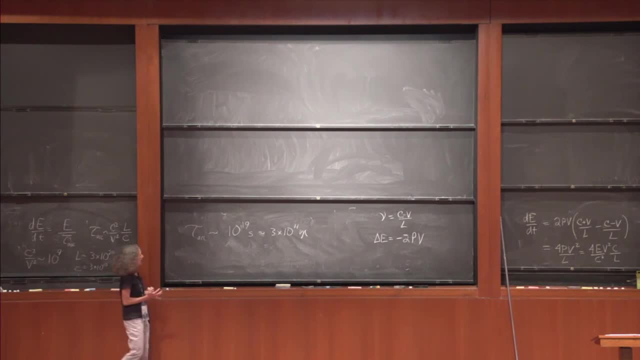 That's the rate at which interstellar turbulence can accelerate cosmic rays, And we know from observations that the lost time is about 2.6 times 10 to the 7 years. So what Fermi accelerators do is they say that the acceleration is about 10 to the 10th centimeters. 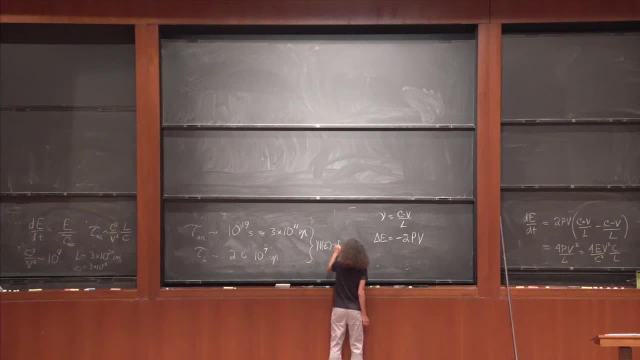 And what the acceleration predicts is that n of e goes as e to the minus 1, plus 10 to the 4.. OK, So very, very steep spectrum. It can't work. The only way to make this work is to make the clouds much. 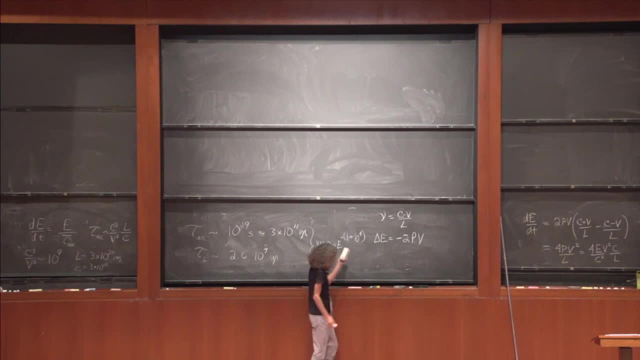 closer together Or much faster, The light element composition comes out wrong anyway. OK, So in our corner of the universe this type of Fermi acceleration doesn't work, And a useful thing to remember is that this is called second order. This is called the Fermi acceleration because the speed of the scattering centers appears. 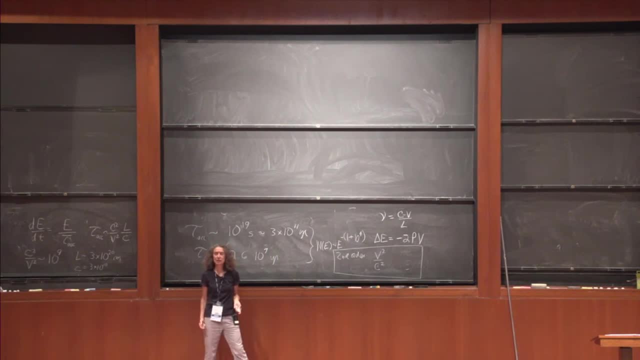 to the second power. OK, So Fermi acceleration, lovely theory, might work in solar flares. Doesn't seem to work very well for galactic cosmic rays. But there are you know sort of serious grown-up models for second order Fermi acceleration. 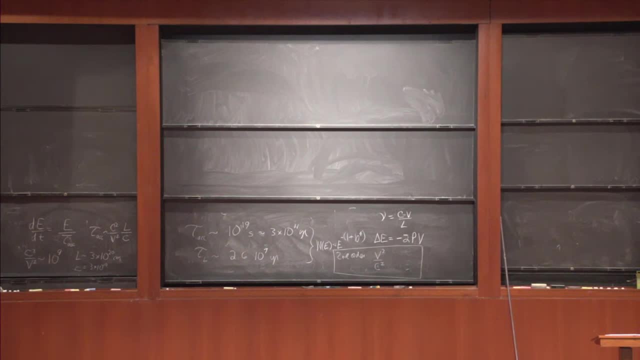 in galaxy clusters, A completely separate problem. OK, Questions about that. Yeah Well, so the L that we chose is about the observed value. It's about 100 parsecs. So to make these two about the same, we would have to reduce L by about a factor of 10 to. 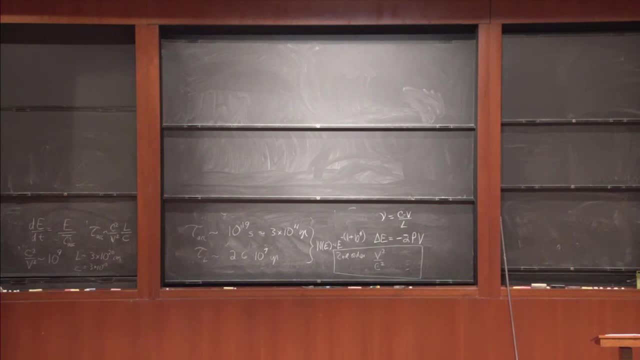 the 4. In other words, we'd have to make it about 0.01 parsecs. OK, That's a good one. OK, And it's for our interstellar medium. it probably doesn't work. The velocity correlation length seems to be much longer than that. 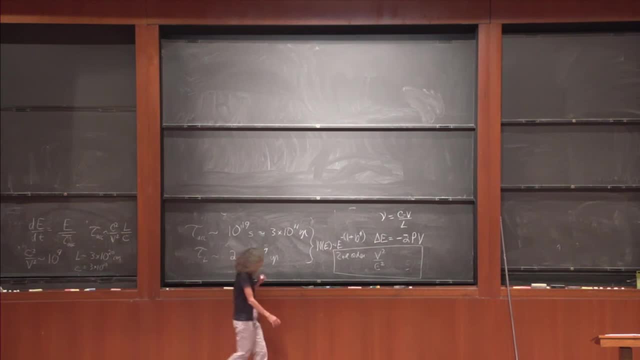 But it might work. Might work in other situations, OK, So, um, So now let's go back to the first equation. OK, So now let's start talking about diffusion, And I can see that I prepared notes for this lecture that are just way, way too long. 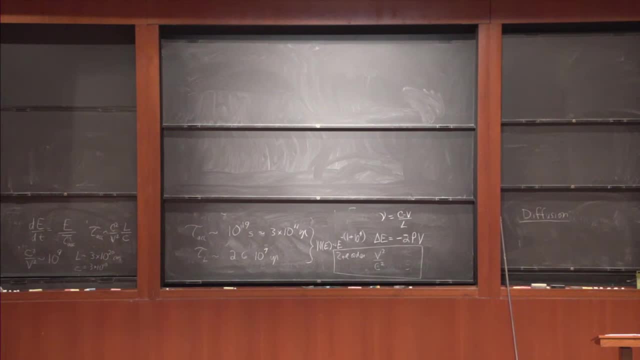 So I'll try to get feedback from you about whether I should be going faster. Should I be going faster? No, Yes, OK, When I teach a class, I have to. if I ask if I should be going slower or faster, I put: 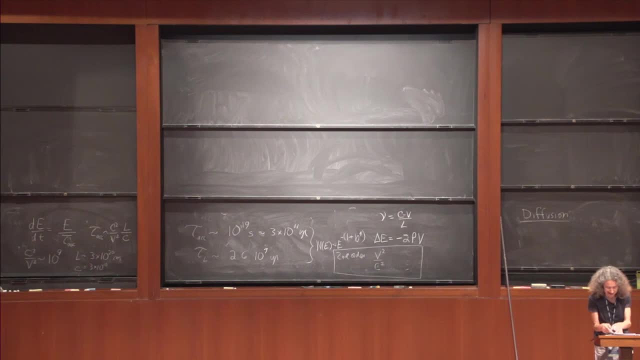 a bag on my head to get honest answers. So let's start talking about diffusion, And we're going to be. what we're most interested in is this pitch angle scattering, And the standard notation for the pitch angle is mu, which is also sometimes used for magnetic. 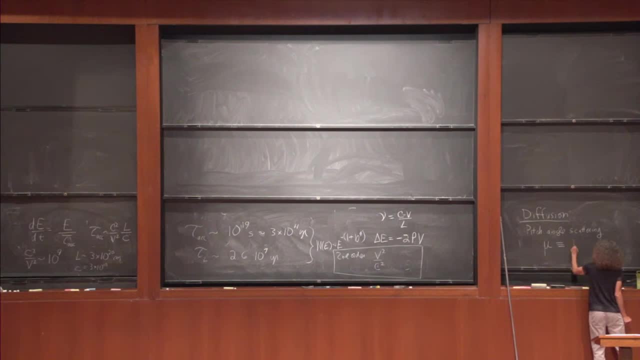 moment, But here we'll use it for pitch angle, And it's defined just as the momentum dotted with a magnetic field divided by Pb. OK, So that's our pitch angle scattering, And let me just say briefly where we're going on this, because we won't have time to finish. 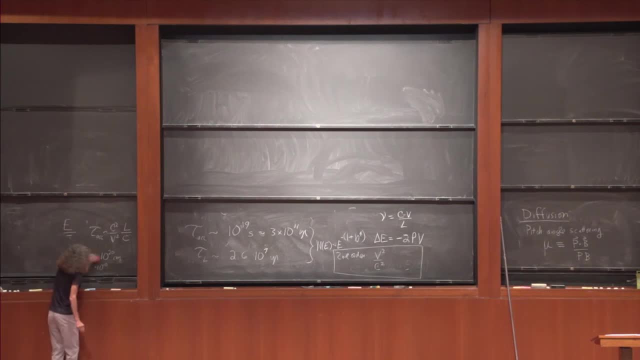 We're going to build a very nonspecific model of diffusion due to pitch angle scattering, So we're going to derive a diffusion in mu space- OK, OK, OK, OK, OK. And then we're going to have show that it leads to diffusion in x space. 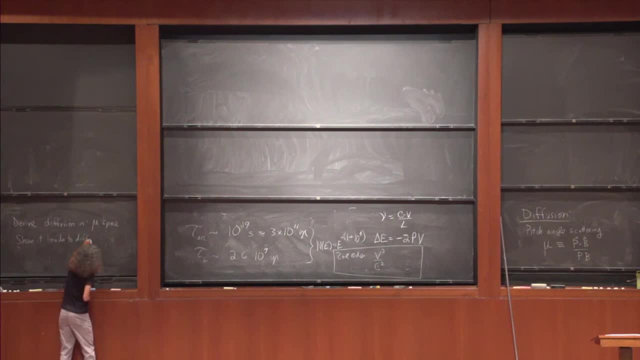 And then, once we have that, we're going to apply it to shock acceleration. OK, Oh, OK, OK, OK, OK, OK, OK, OK, And then we'll worry about how to make it self-consistent. So the general idea is the same as it. 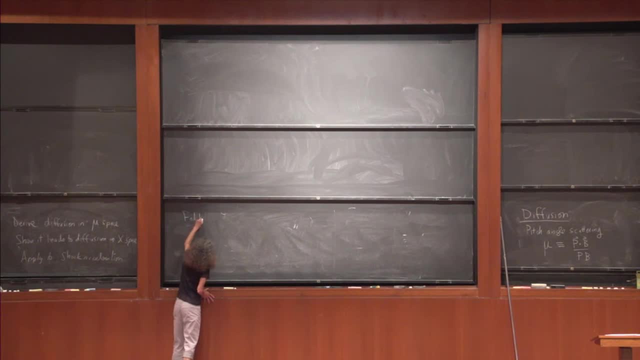 is for all Fokker-Planck equations. How many of you have seen these like in a stat-mech class or a plasma class? Lots of you, Great. OK, So we're going to derive a probability function, at risk of confusing it with momentum. 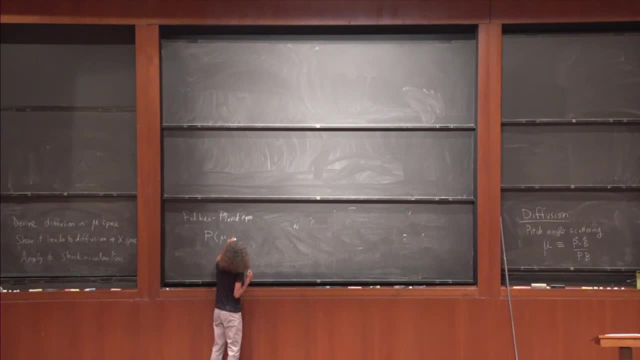 So p of Mu and delta mu will be the probability that a particle with pitch angle mu is scattered by some amount of delta mu in a time delta t. I think that's the way I wound up defining it in the end. Yep, OK. 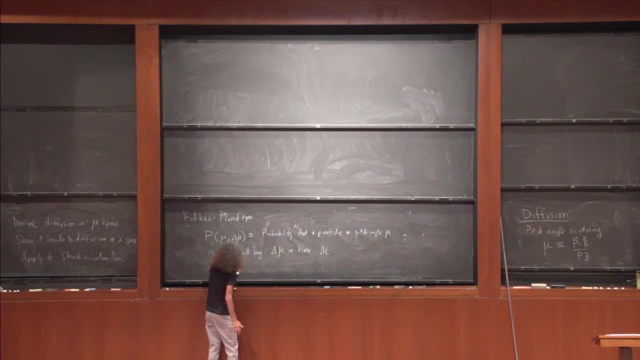 So we have a, and let's assume that we have some normalization such that the integral of p of mu and delta mu integrated over delta mu. let's just call it some number c, It won't matter what it is, And then we have a particle distribution function. 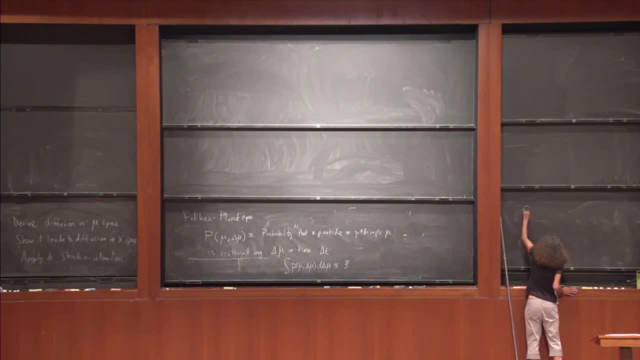 So f of mu and t is our cosmic ray distribution function, And of course it also depends on position and momentum, but we're going to just suppress that to stave writing. So f of mu and t plus delta t is going to be what? 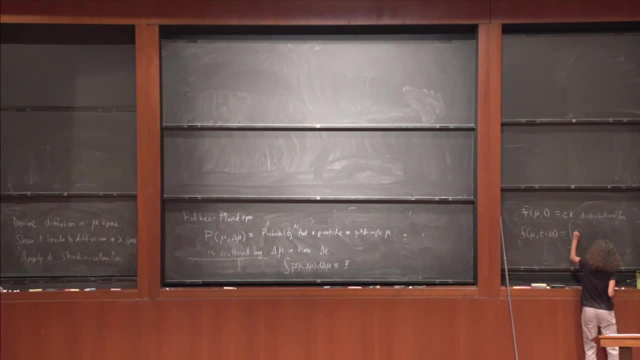 It's going to be the integral of f of mu minus delta mu and t times del t, What vt times p of u minus delta mu and t d delta mu. So these are all the particles which can contribute to being mu later on weighted.